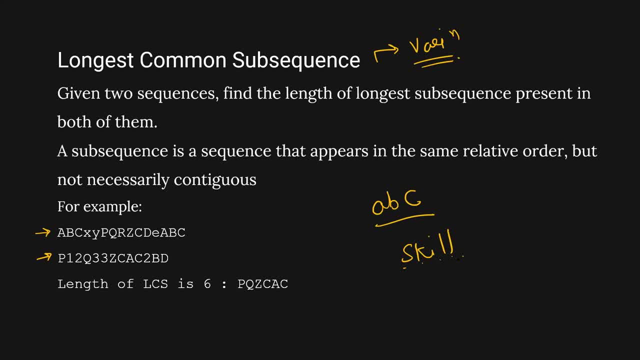 let's say skill. So S K I L L. they are in sequence. But when I say subsequence, S I L or A C D, A C D is a subsequence of that. or S K L or S I L, These are the subsequence. 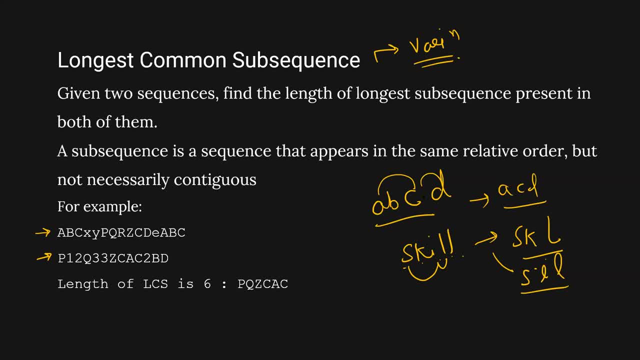 of different length. So what we need to find it out. So, out of all possible different subsequences of these two strings, let's say what is the longest such? So longest, with just logic of ours, mathematically, we can find it out that okay. 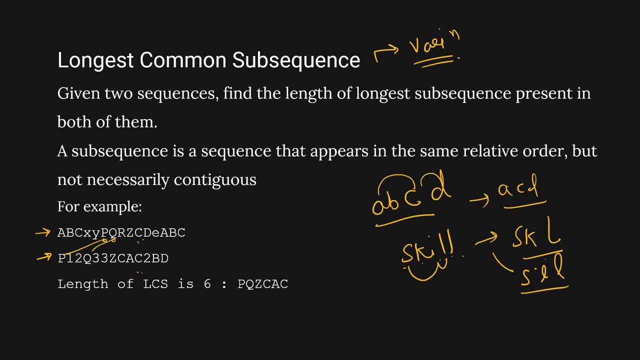 hey, the P and P are matching first, then Q and Q are matching first, then Z and Z are matching first, then C and C are matching, then A and A are matching, and then this C and this C are matching. Okay, 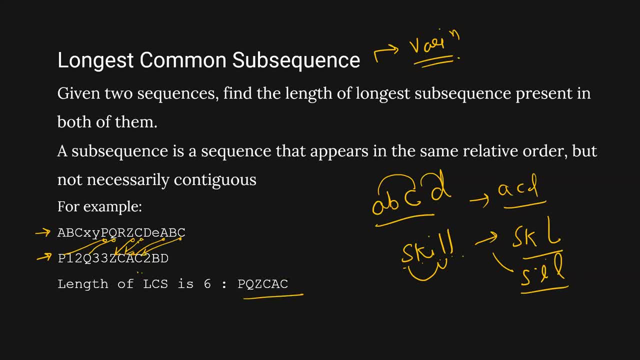 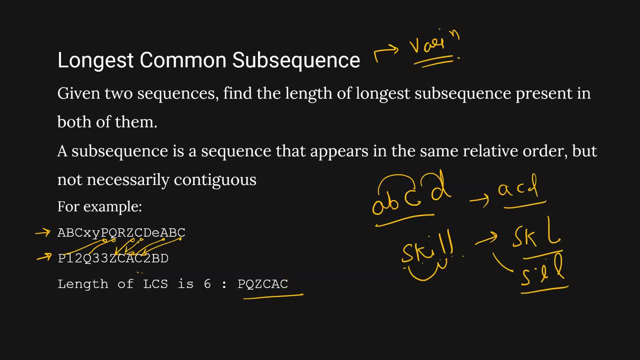 Okay, Okay, Thank you, Thank you, Thank you. Okay, Okay, Thank you, Thank you, Thank you, Okay, Thank you, Thank you, But when we have to program for that, how we can find it out which type of interview questions? 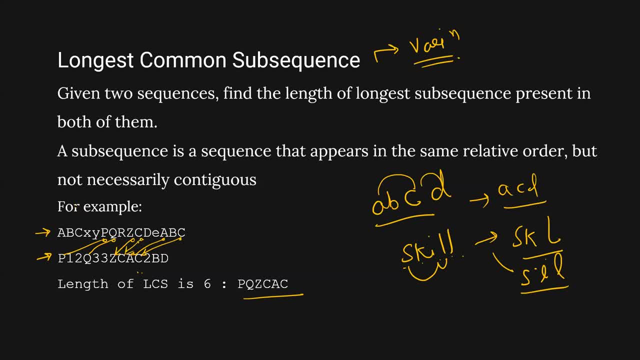 can be asked Obviously directly. they won't ask you the longest form and subsequence. What they will ask you is: let's say you're writing a code for DNA matching. Then find it out if this two DNA sequence are matching more than 80% or not. 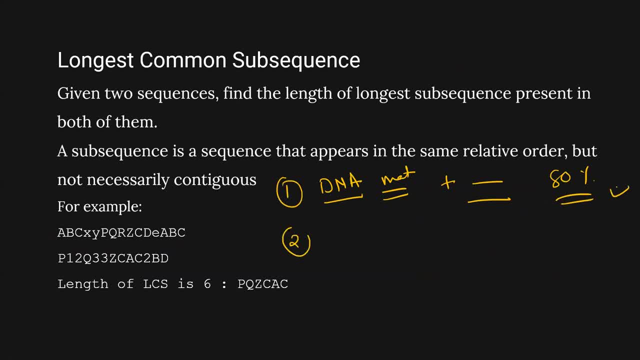 this is one type of interview question. second type of interview question with this can be that if we have a tree, oh sorry, a river, and over here the docs are arranged, doc numbers are arranged in different order, right, let's say one, six, three, nine, eight, and over here eight, six, one, three, nine something. 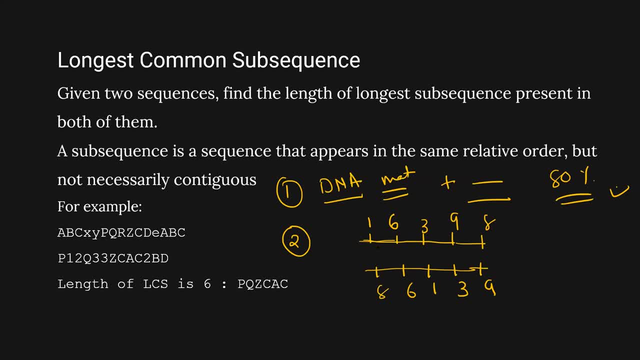 like that. now, if they can be only connected like this, one to one or six to six- let's say we want to create a bridge on that- then what is the maximum number of bridge we can create such that they will not overlap? so one, two, six and six to six, if we create they will overlap. 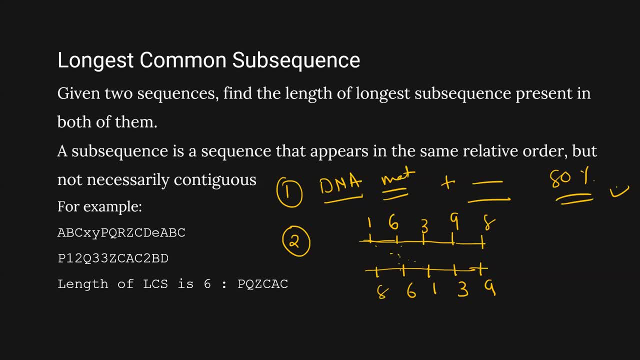 we cannot create a bridge on this one, two, one and six to six. we can create only on one. then what is the maximum number of bridge we can create? so if you see it's a maximum sequence between these two, correct maximum lcs between these two strings. so in that way, some modification of lcs. 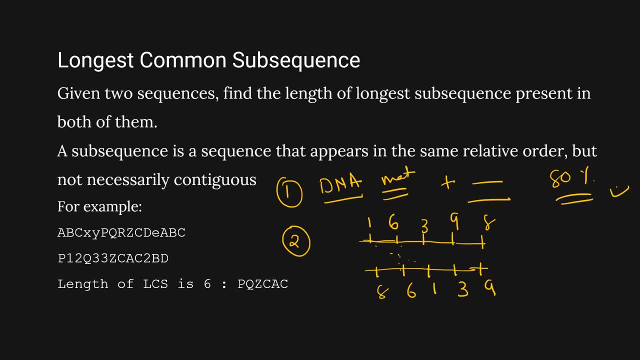 will be our in interview, and then you'll have to apply a logic to find it out. the solution makes sense. so far, any doubt. now we'll see how to think in this dynamic programming. dynamic programming is one of the toughest topic of all in interviews, so that's why i have chosen to give you an. 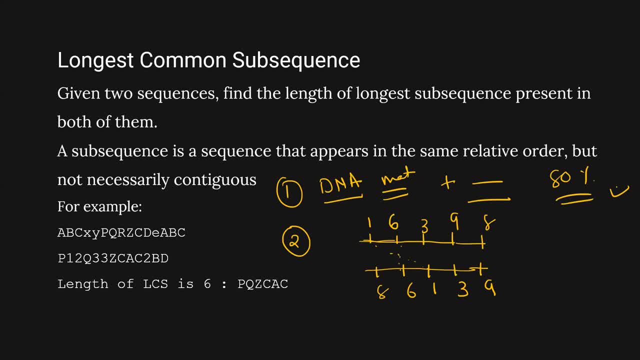 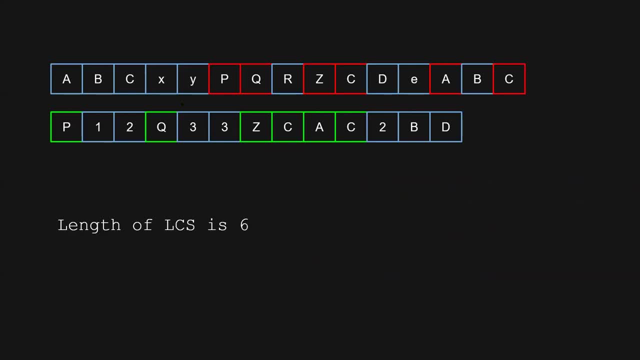 overview of how to think and not to fear from tp. let's see. so we know that. let's say, for this sequence, these two sequences, the largest lcs is six and how to find it out that. so, with just a smaller example, we'll try to create logic for that. so first our 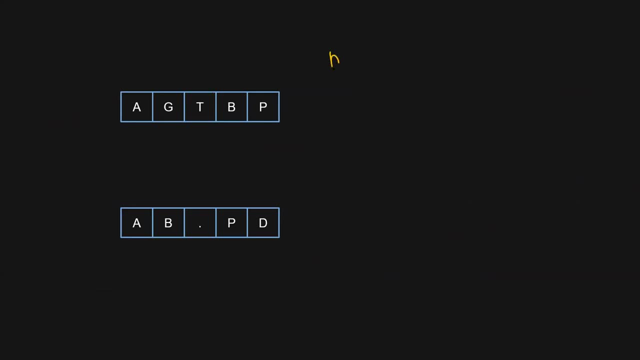 mind will always see that can we create a brute force solution or not? like i'll always say, my mind will always see a problem and be able to solve that same problem. that i possibly will do, because, with my mind, what operation can i use with just the lcss yours like? 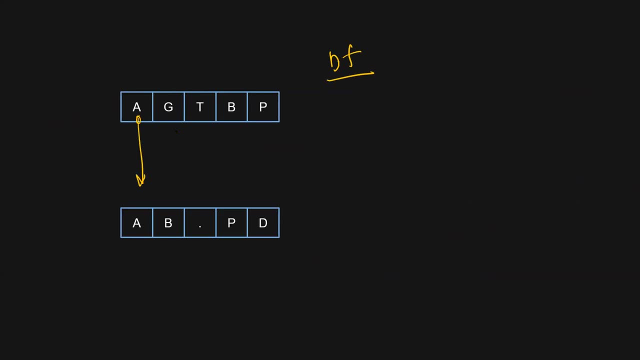 i'll. i'll search from a to a. if it is matching, then i'll move for g to a, g to b, g to dot, g to p and g to p and g to d. if it is not matching, then i'll go for t and then furthermore, and then i'll. 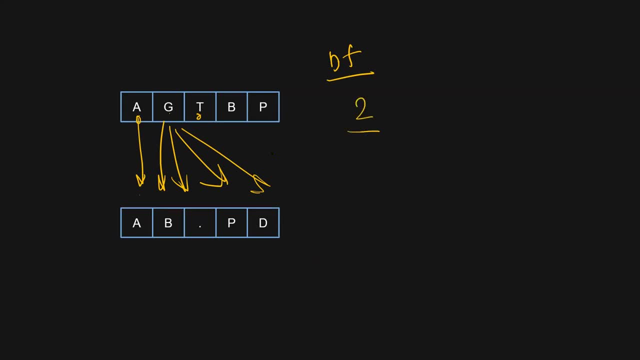 find it out. so for starting with a, i have two lengths, substring which is matching. then starting from g, something else, starting from t, something else, starting from b, some other number, starting from b, some other number, and i can get the result like this. so in a brute force way you can find it. 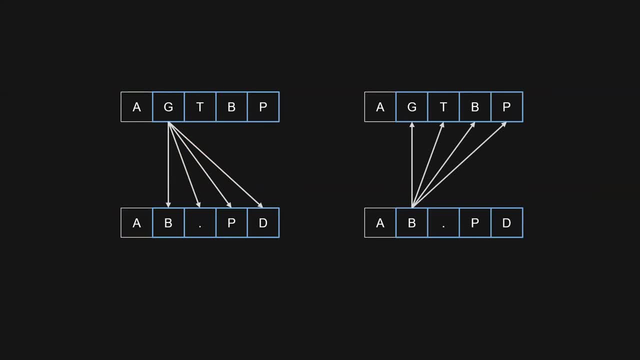 out correct, but how complex the solution will be. brute force way you are matching, like in order of n square, you are matching each with each and that two multiple times, starting for a order of n square time. starting for g: order of again n square time. starting from p: again order of n square time. so 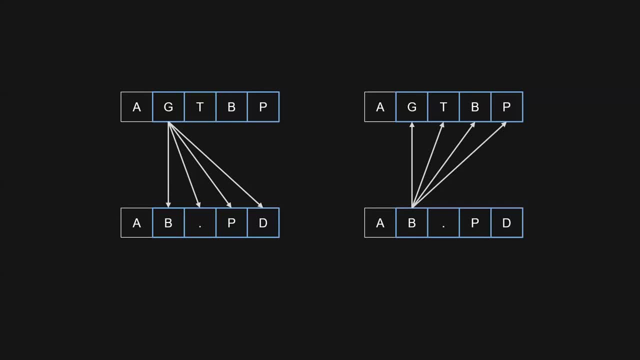 it will be more than order of n cube. i would say in typically order of n cube only, but for further other compute, computation if you do, finding out or storing it into hash map and all that things, just for you know largest number, and all that things. if you do, furthermore, the complexity increases. 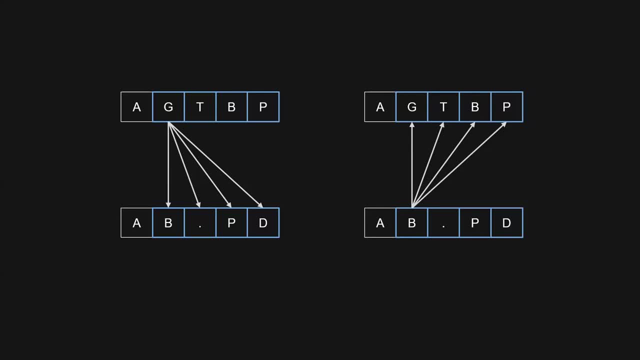 with a brute force solution, what we can do to further optimize the solution. how should we think so generally? we should always think, probably, if you remember, in college days or school days. we have a theory in mathematics that if a theory can be proved to be true, then we can. 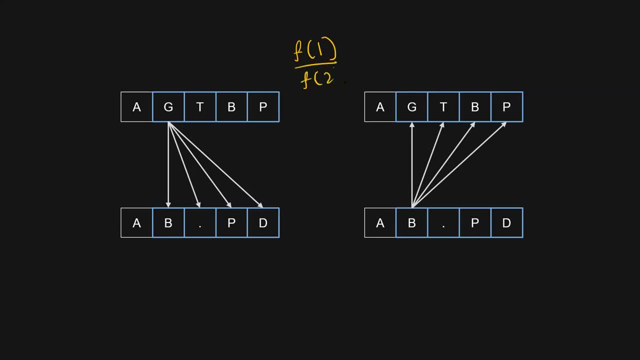 prove it for f of one, which is the smallest number, f of two, which is another next smallest number, then for some arbitrary number, f of n. if an equation can be proven for this three, then it can be proven for f of n plus one as well, and that's why for any f of t it can be proven. 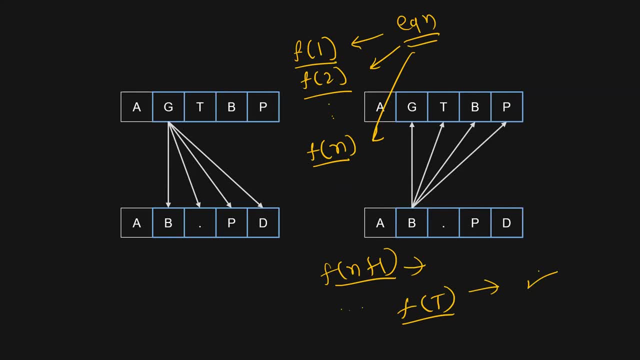 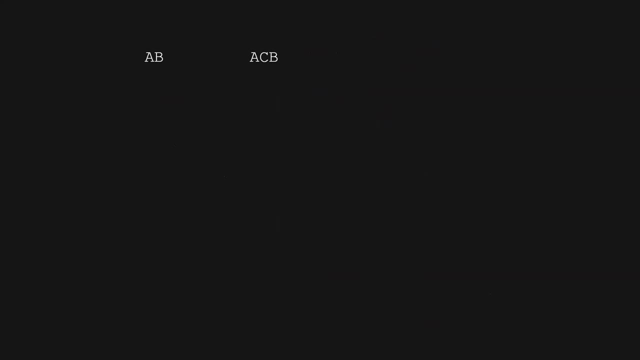 same mathematical phenomena we will apply over here in dynamic programming almost everywhere which is related with strings, and we'll try to build up the solution. let's see how, what a smallest such substring we can find it out is with two or three characters. a smaller strings we can find it out with two or three. now let's try to apply. 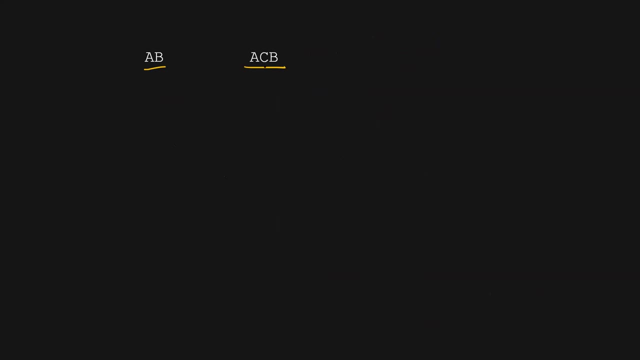 a logic in that. let's say, if we have just two sub, uh, two such strings, let's say a, b and a, c, b- how we can find it out the maximum common substring between those? we see a and a are matching. this our first logic, then what we think is okay if a and a are matching. 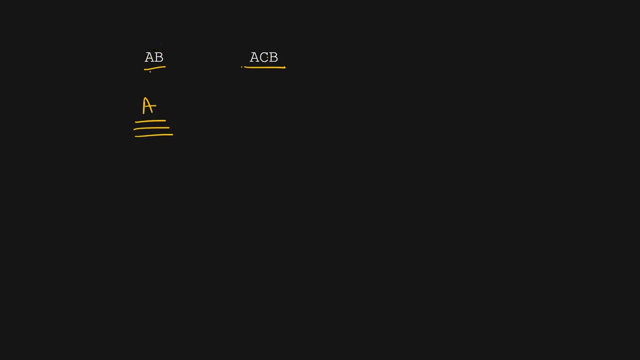 then again, just like a brute force method, i'll see that rest of the elements in b and c, b, how much they are matching. or from b and a, c, b, again how much they are matching. what is the longest common substring subsequence in this? just manually we are thinking that gives us idea that what if there are just 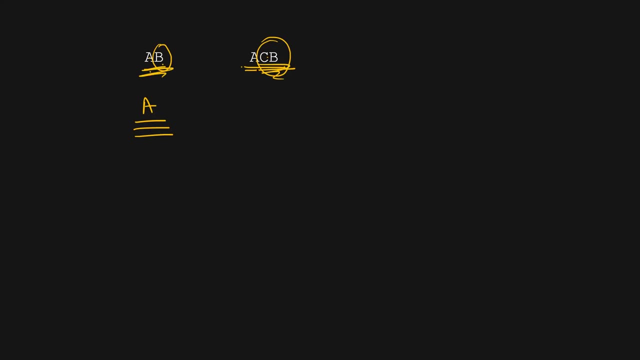 two characters or three characters over here, then what will be in terms of coding logic? so so far we have thought in terms of mind or in terms of, you know, logical argument. now we'll try to convert that logical argument in a base case of a recursive solution that, if we have just a very smaller 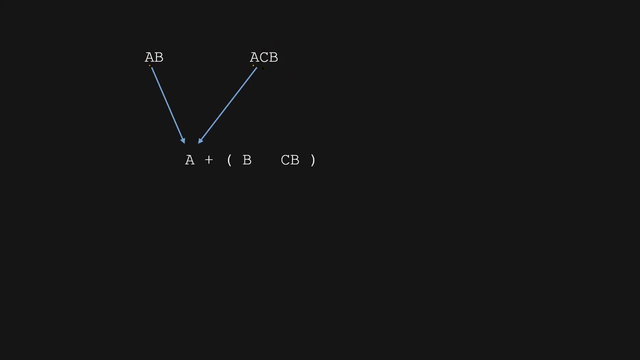 string. then what we do? if first character of these two are matching, then we'll say, okay, a is matching. then in the rest of the strings, b and cb, how much common characters, in increasing order, are there? so our problem: from a, AB 2 length and ACB 3 length is reduced to 1 length and 2 length. 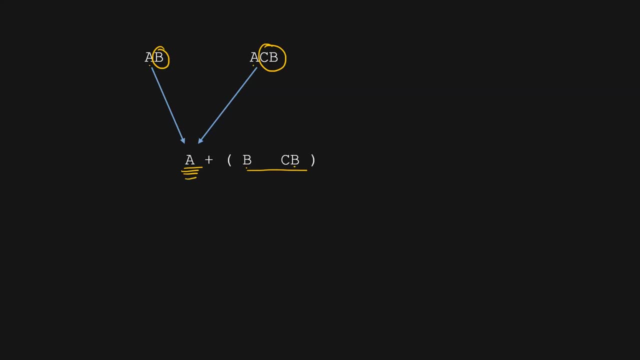 Now that's something programmatically we can do. Now what if first characters are not matching Obviously? let's say, first characters are not matching PB and ACB, something like that. So if first characters are not matching, then what do we think logically, 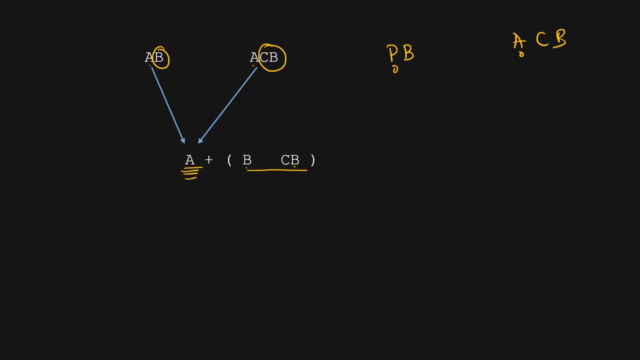 Well, that we don't know rest of the string over here yet. We don't know rest of the string over here yet. Then we think that there can be two possible ways. One is that if P and B and ACB are not matching, then what I'll do? 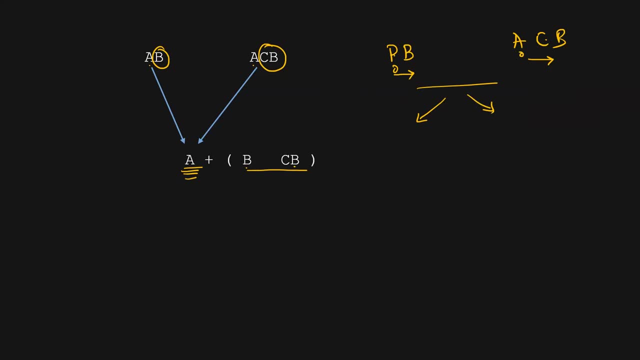 Obviously P and A will not be part of my common subsequence because they both are not matching, But they can be matching in rest of the strings. Let's say PB, AC, B, something like that you have in future, In future, in the sense, in rest of the string, we don't know. 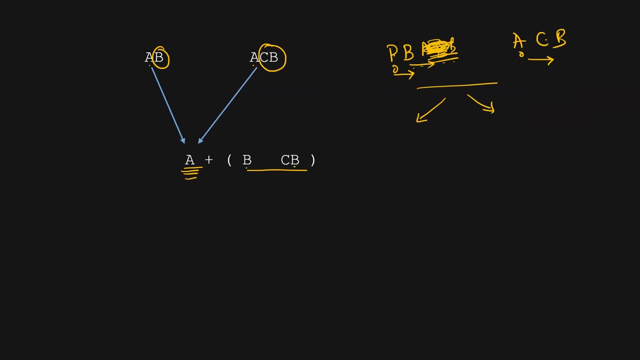 Then what you think is okay, I'll search, instead of P, rest of the substrings B and rest of the substrings if there are ABC and some with ACB as it is, in case they are matching. So at least you are reducing one string's length. 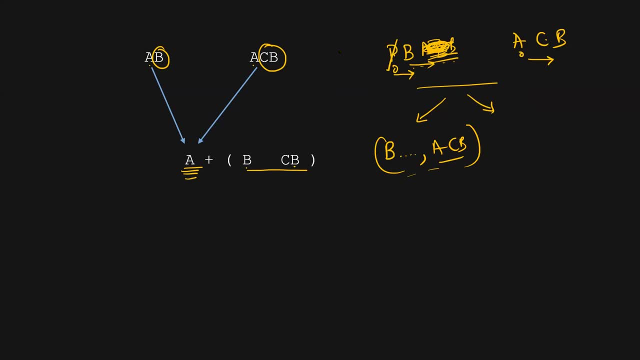 as in a subproblem. So from a larger subproblem of N strings and M string we have reduced to N minus 1 and M length string, And the same logic will apply. What if P is not part of subsolution? then this can be there. 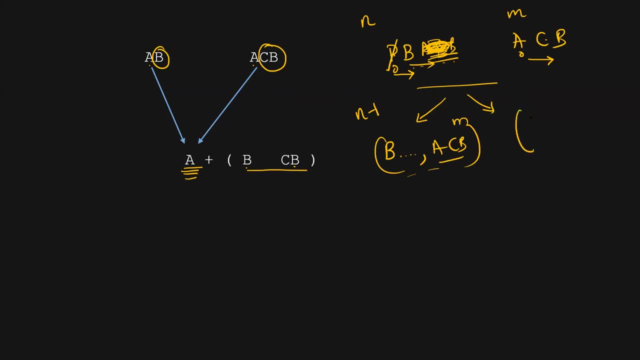 But if A is not part of subsolution, so what you'll do Then for rest PB and rest number of nodes, or whatever number of characters A doesn't come, then in CB how much they are matching we'll see. 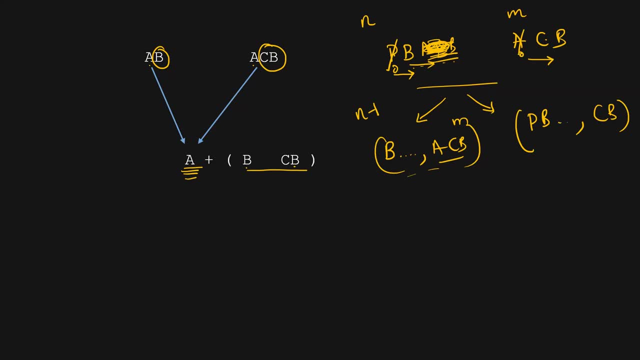 Okay, so logically, recursive solutions to create recursive solution that is created, how programmatically it will come. that is first thing. Second thing: will it solve my problem? Third thing: what will be the base cases? What are the base cases for that? 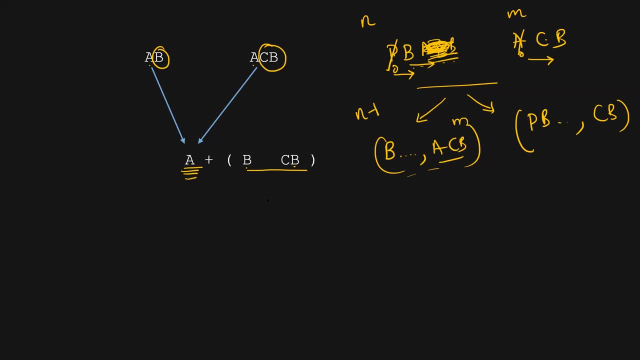 So let's think about the base cases, that if there are, what is the base case? The base case is something like this: If there is only one character in the base case, if there is only one character in the base case, if there is only one character in both the strings A and B. 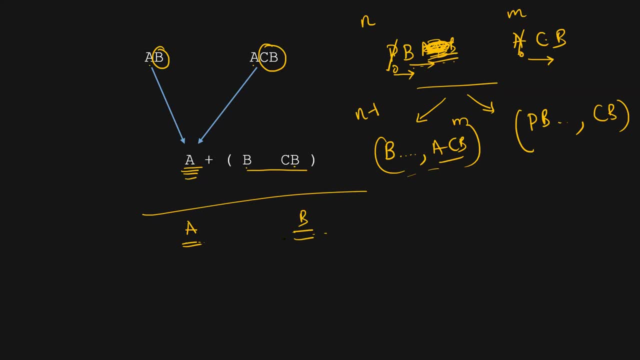 we can directly check whether they both are matching or not. If they are matching, I'll return 1, because it's a recursive sum. let's say I'll return 1.. Let's say they both are matching, then 1, like this: 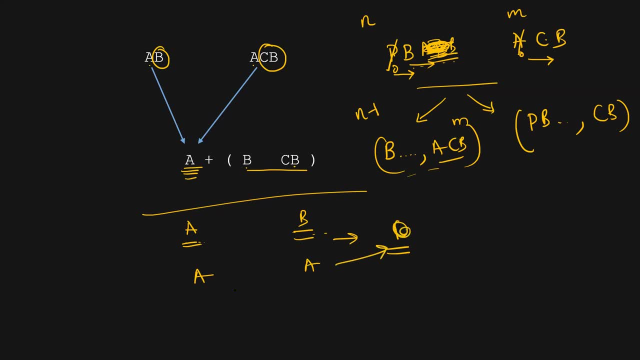 If they both are not matching, I'll return 0.. Let's say this is first base case. Another base case can be that if there is only two characters, AB and BC can be right or wrong. one of the string can be right or wrong. 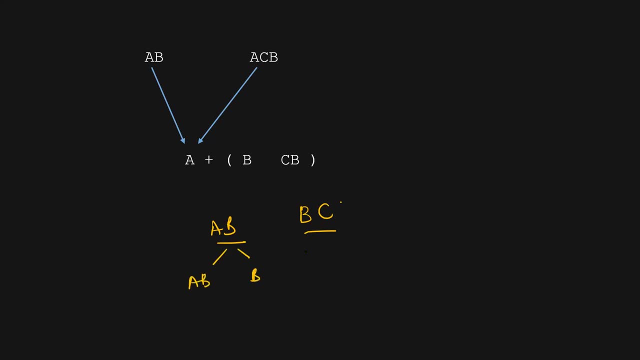 right if there is only one character in one of the string, or both the strings Right. then again I can divide it like this: AB, B or sorry, AB and BC. two character strings are. I defined it something like this: A and DC or B. 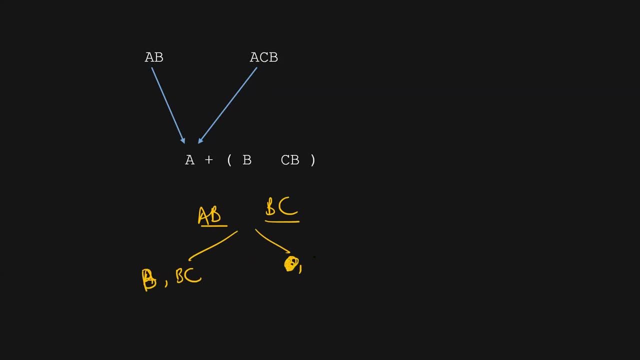 Sorry, B and BC Or AB and C, Great in one of the string, Great Two characters will be like that. So how do we do that? and c first, first character remove. now again i have just one character. i can again move further. 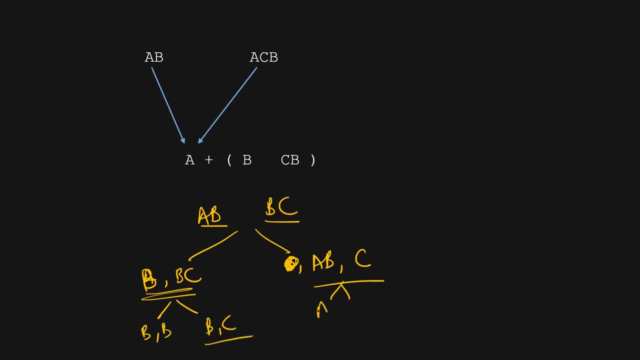 b and b or b and c, or a and c or b and c. now over here i can directly with until a last part, where f of length is one. if i can prove that over here it will return one to its parent, it will return zero. so over here i can define that. what is the maximum of common subsequence in b and b, c? one. 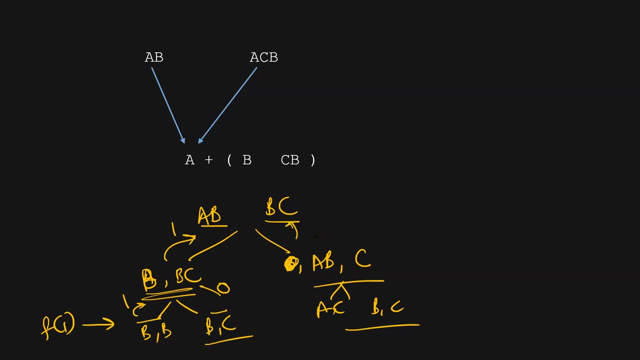 that i'll return to my pair and over here also, i'll return the same value to my parent. and a, b and b, c can define over here sub problem can define that. okay, maximum you can get is one which is either, which is b, b, a subsequence, and it will give it to its parent. so we see. 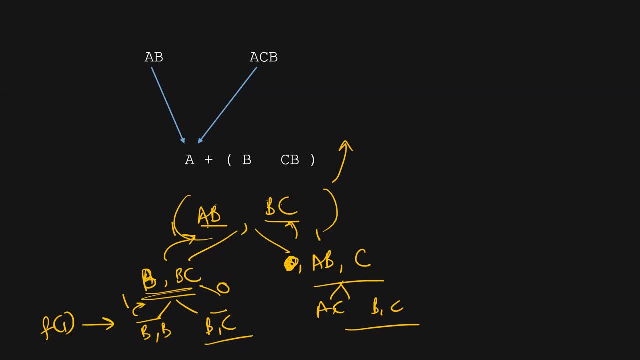 we created a subsolution at the level one with the least number of characters, in that that we propagate it for larger level or larger length of strings, and that obviously is getting propagated towards the upper. that means more number of strings. so such way i think we can create it. so, as i said, 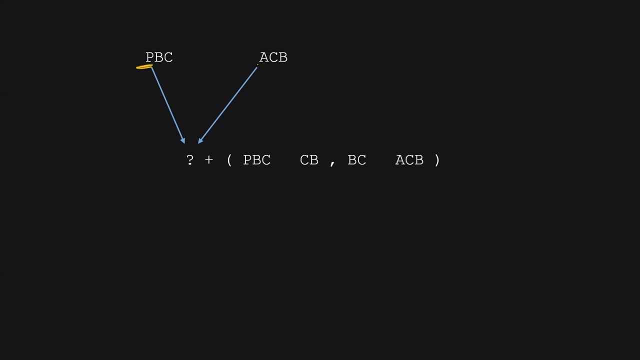 recap: if the first characters are not matching, then what we do? okay, the whole string can be matching with rest of the string. if a is not part of solution, or if p is not part of solution, then rest of the string can be matching. so again, we are reducing my problem: its length from nm. 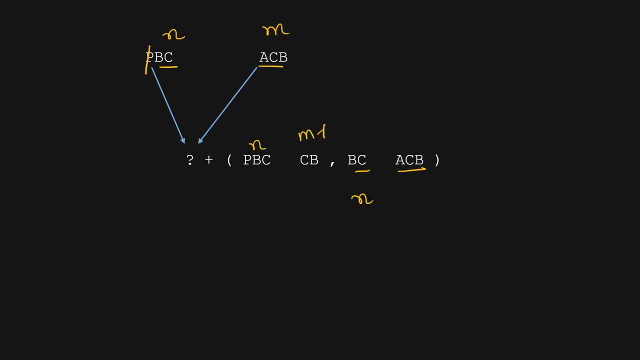 to nm minus 1 or n minus 1 m, and i'm moving further recursively. i'll try to solve the problem over here. got it? so now we understood that. okay, recursively i'll have to solve lesser number of length until one level of length comes of the string and i can return whatever the 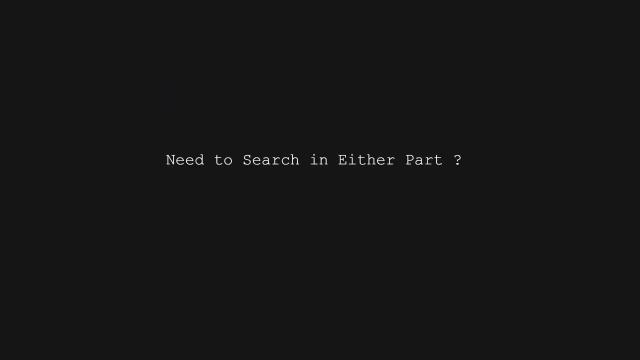 maximum matching of characters are there. this is further more examples with larger strings. so if you see recursively, if i create it can be like this longest common subsequence with string one: string two: i is a starting index of s. j is starting index of string two. length of string. 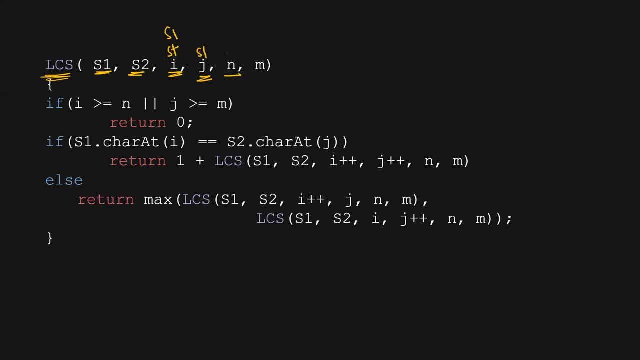 one. so it's a starting index of string one, starting index of string two. length of string one and length of string two. that is what is defined now in recursively, what we are trying: finding it out whether the first characters are matching or not. that's what we're going to do, and then 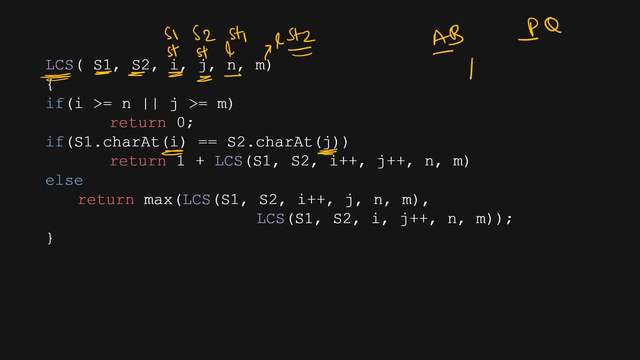 doing right. pq, a and p are matching or not. if a, b and a, q p, let's say, if first and characters are matching, what we are doing we are doing for b and q p, we are recursively solving for b and qp, so it's the same thing i'm doing. return one plus because a and a are matching. return one plus. 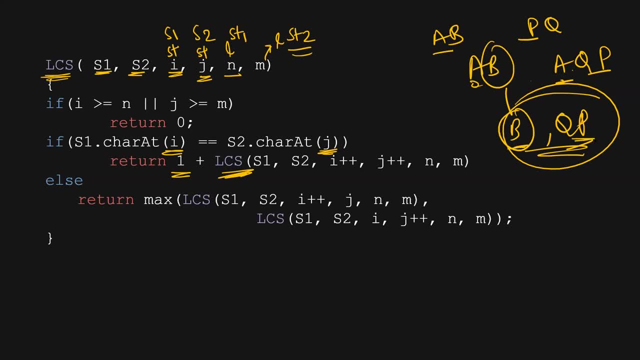 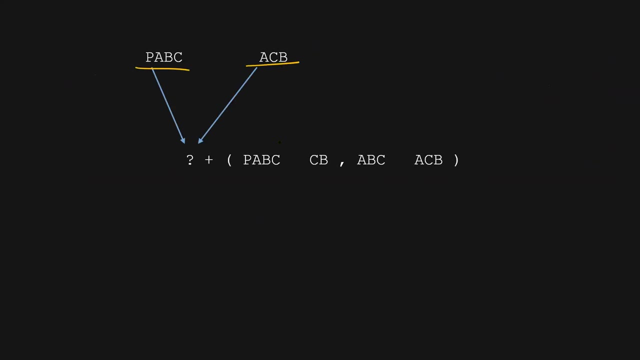 again solve the same sub problem with a string b and qp, which is string one, string two, but its starting indexes are updated. length remains same if they both are not matching just like this. what i do solve for two recursive solution in which the length of one string is reduced and the length of in another one length of other string. 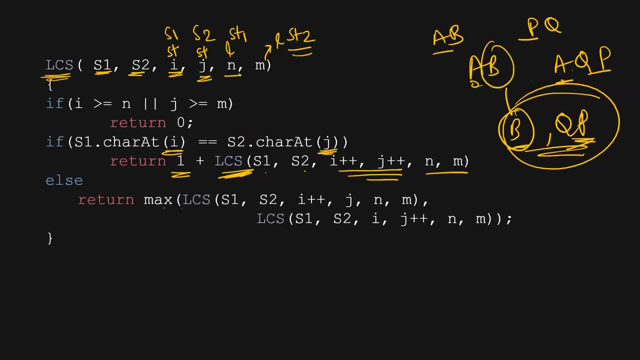 is reduced. so the same thing i'll do: the maximum of, then i'll find it out. whatever the maximum of is true, the maximum of sub problem as cs, string one, string two increase the character in first one. the rest of the things remains as it is. increase the. 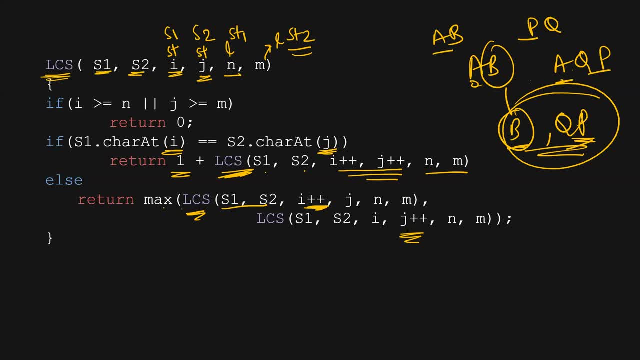 character count in second one or increase the starting index in second one, and rest of the thing remains as it is now. after this recursive sub problem completes, it will give me the result. whatever it will return, it will. it will be my answer, so far clear. now we'll move further. 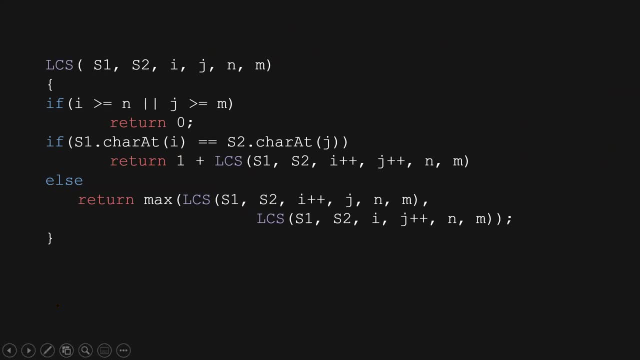 now we'll move further. when we always have to do counties of which series you uh know later on, we can imagine something like this: that, okay, we were matching first character. can we match the last character? yes, we can match. some coding strategies will get changed then how? 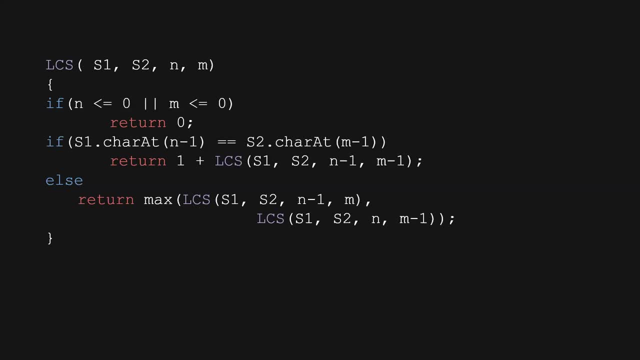 and why do we need to convert it into a different kind of solution, which is dynamic program? so this was a recursive solution Instead of first character. if I'm checking with last character, it can be directly n minus 1, m minus 1, and n? m minus 1, right. 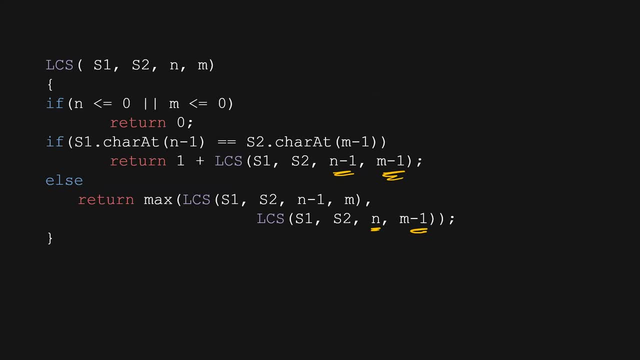 Because I'm checking directly the last character, So I'm reducing from back side. That's it: I'm checking the last character and I'm reducing from back side, So the solution is bit simplified: instead of checking at the first character. 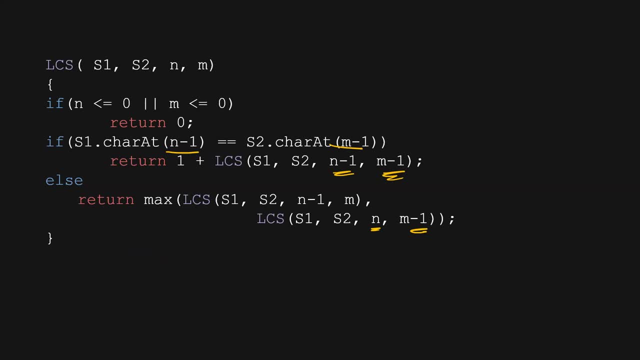 But in both the ways, in both the logic, the solution can be created. Now a point comes- is why recursive solution won't work in more general day-to-day life? Because the recursion itself stores a space in stack. Because recursively you are storing everything into stack, right? 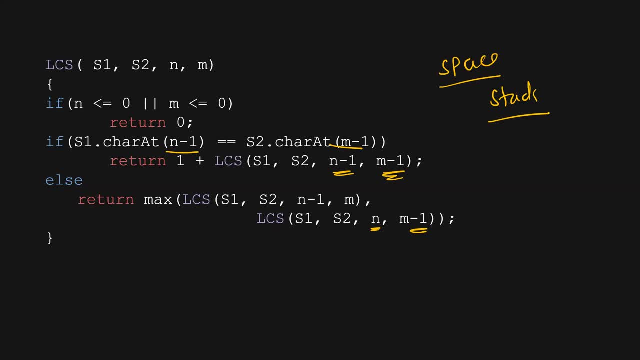 We have seen, like how recursion works Internally, it uses stack. Yesterday we have seen. So internally space is utilized And when space is utilized, your time complexity will also increase, because you are storing everything into space. 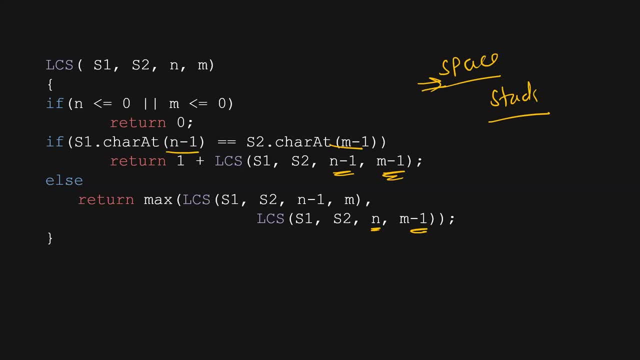 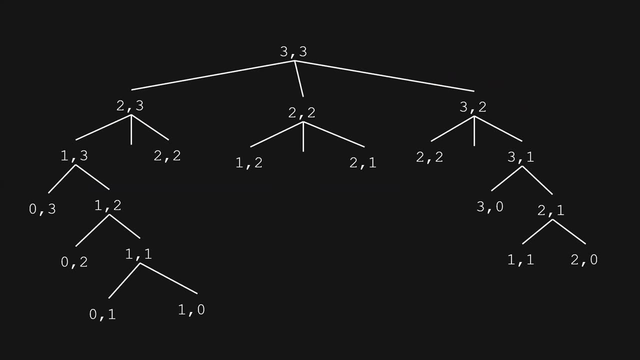 You are taking out the values from space, So that stack time will come into the picture And a same sub-problem you will solve again and again. So let's say, the length of the strings are 3, 3.. 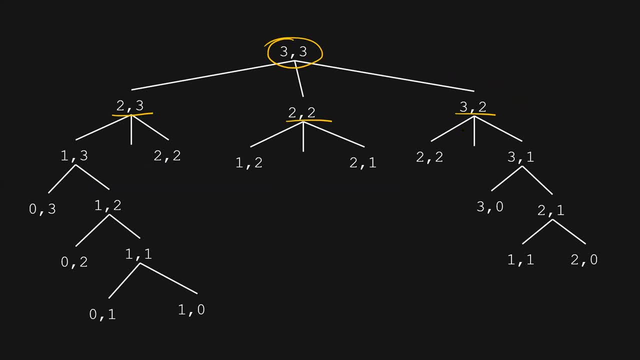 Then you will solve for 2, 3, or 2, 2 or 3, 2.. So let's say 2, 3.. So if you solve for 2, 3,, you will solve for 2, 3 or 2, 2 or 3, 2.. 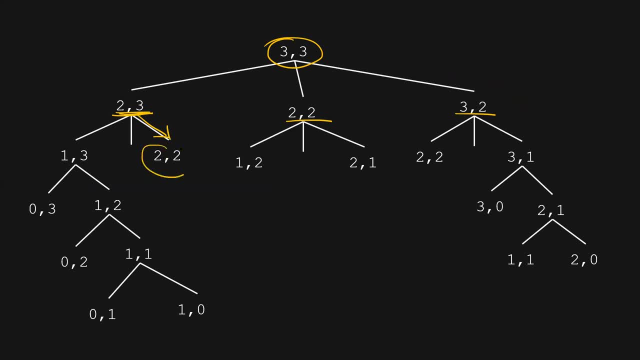 So if you solve for 2, 3,, you will solve for 2, 3, or 2, or 3, 2.. you see, at two, three, again, you'll solve for two. two, that means of length of two, two which you. 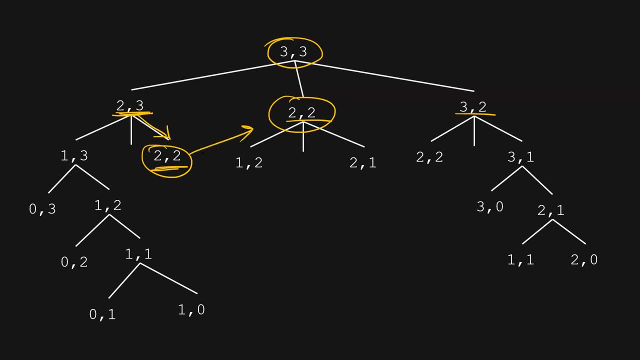 would have solved over here as well. so the similar sub problems. if i give an example of this, let's say a, b, c and p q r are there, or p a, b are there, you would have gone for this as well, gone for this as well, like a, b and p a c, like this, and over here, three length: a, b, c and p a as well. let's say: 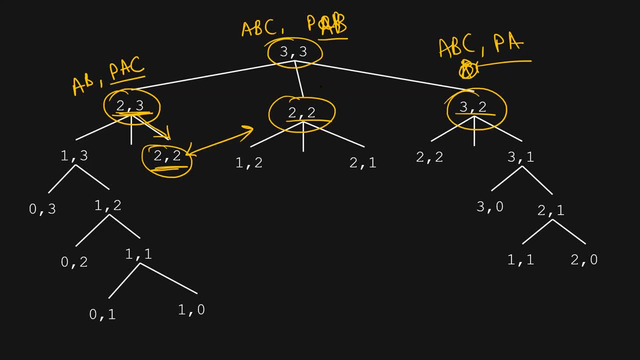 got it now over here. what will be the sub problem? probably, if you go for two, two then it will be like b, c and a c. so same will come over here here: b, c and a c. got it. so same length of or the same type of sub problems you will solve. 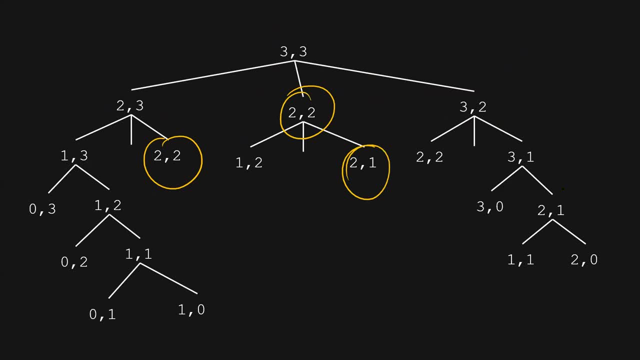 again and again something like this: two, one, two and two, two is again over. so, in order to reduce the recursively solving the same sub problems again and again, what we can do, can we store the results of this so that when we compute this at that time we can see whether it's already been? 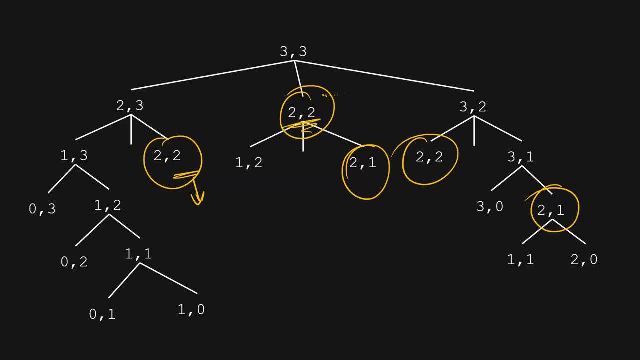 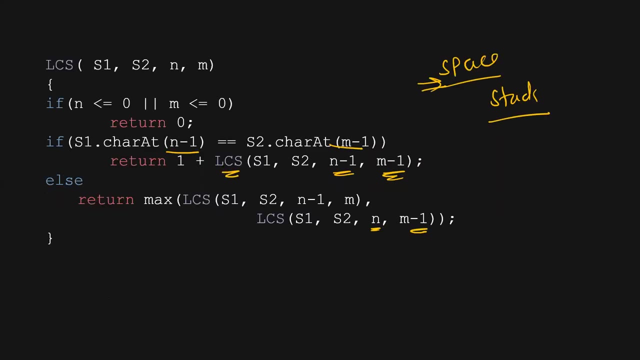 stored or not, whether it's this is already been, this recursive formula or recursive thing is already solved or not. so how can we do that storing a result? so in recursion, if you see there are four parameters necessary in this solution over here only two parameters are necessary in. 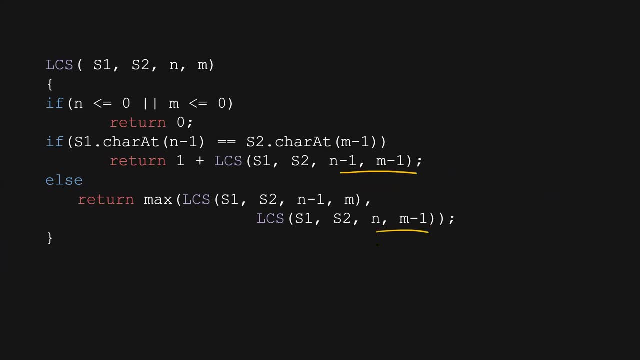 this solution if i store in some way that the solution for this recursive parameters- these are constant ones, so that's why i'm not worried about this- s1 and s2 strings- but indexing, which is i'm worried about. so if for this sub problem, if it's already been solved, i don't have to solve it again. 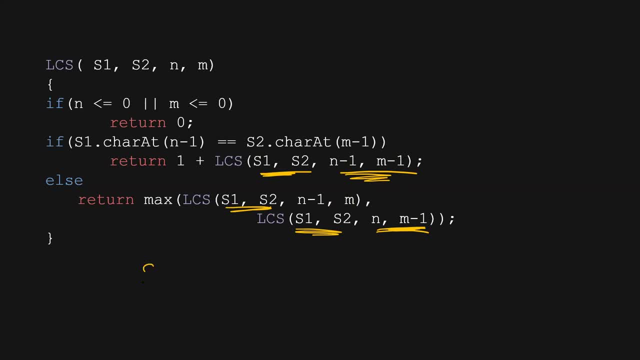 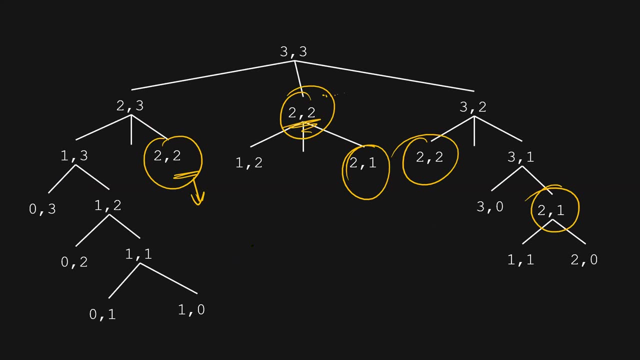 so what i do? as there are two parameters, i need to create 2d matrix. so if i store a result of this, let's say if i store something like this: 0 1, 2, 3, cross- 0 1, 2, 3. 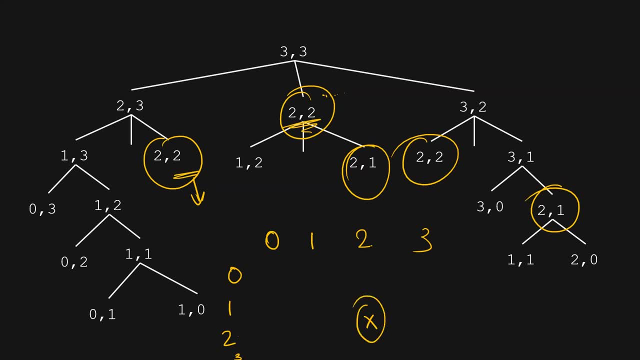 a 2 cross 2 value over here will have a result. so before recursively calling this, i'll check whether the 2 cross 2 in my result 2d matrix is already solved or not. if it's already solved, i won't call this, so that i am reducing number of recursive sub calls. 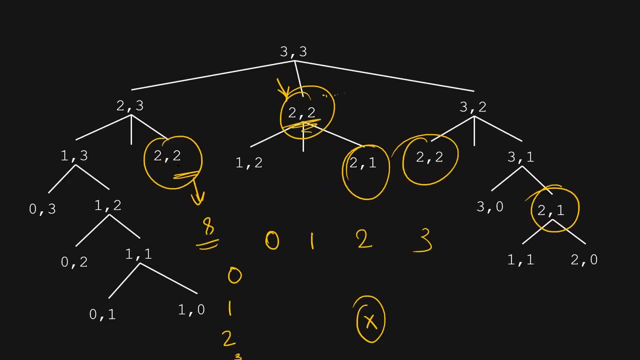 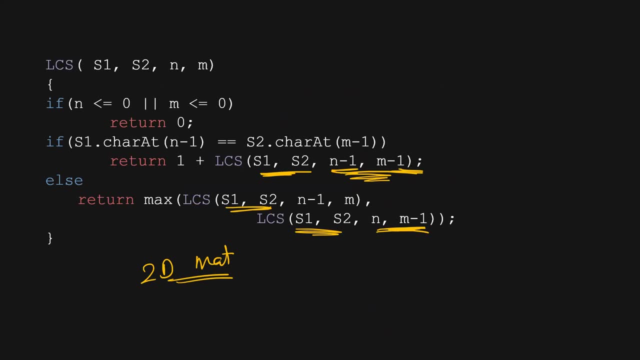 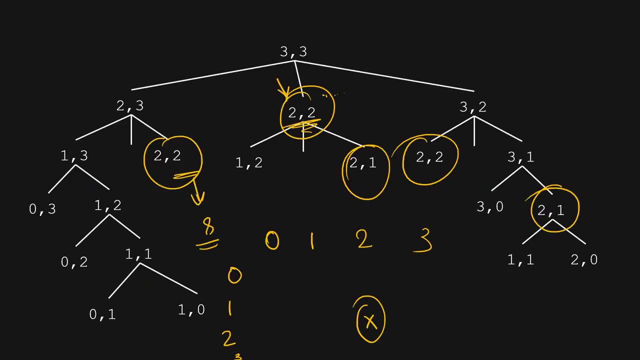 i have to store and what this 2 cross 2 means. this 2 cross 2 is, this index is simple, so each indexes or the combination of indexes will give me its result in a fairly and simplistic way. so in a simplistic way if i convert it into dynamic programming it. 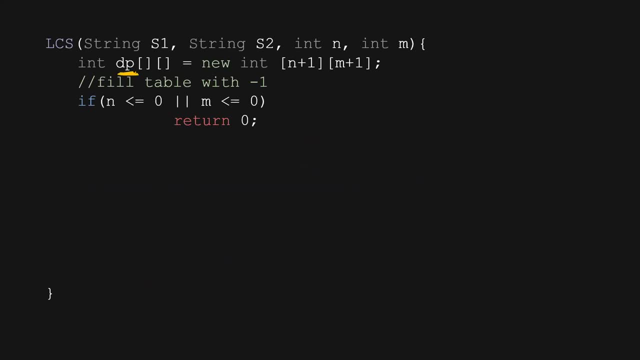 will give me a solution like dp. i'm creating a dp table with n plus 1 and plus 1, just like this: 1, 2, 3- and what i'm doing is i'm storing the result. if it is not stored, first thing is that 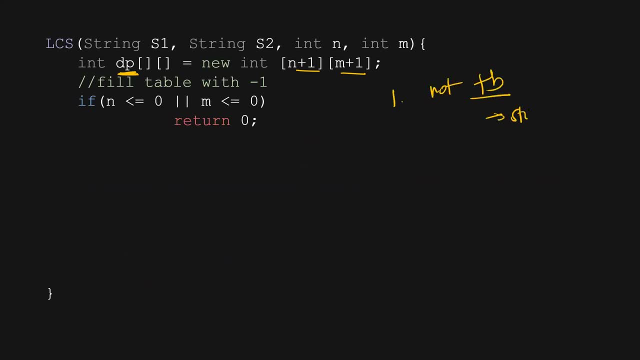 if it is not stored into table, store it. and second thing, if it is already there stored, return it. that's it. so if i convert, it can be converted like this, that if first character numbers are the last character numbers are matching right, then return the value of dp table, which represents n minus 1 m minus 1 dp of n minus 1. 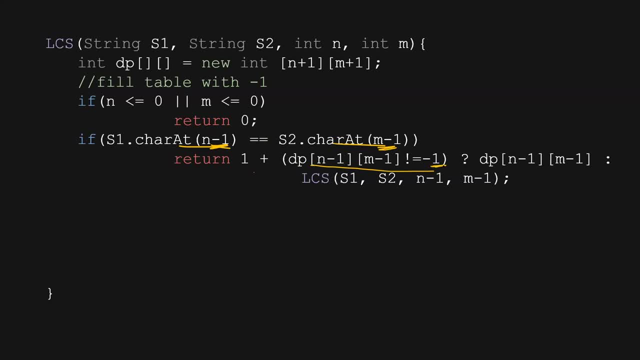 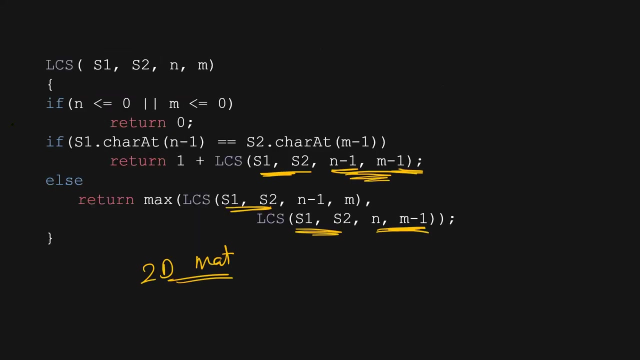 m minus. if that value is not minus 1, that means it's not. if it is computed, then return the value. if it is not computed, compute it. when you compute it, you need to store as well. so first we have solved for. if now we'll solve for else in the same way, and then we'll do what, 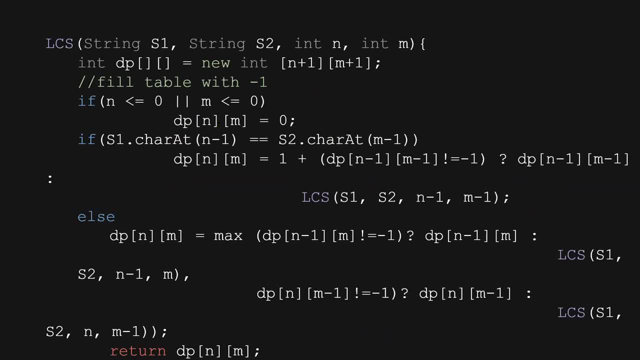 we need to do in the same way and then we will store it. then we will store it. so if the characters are matching, we'll get the result. if it's not computed. if it's computed, return it. if it's not computed, compute it in the same way. in else part, also the same thing. 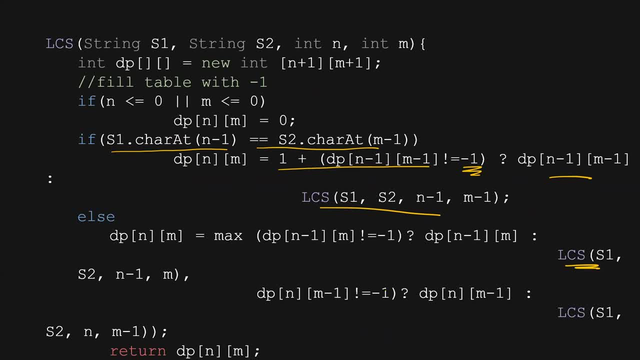 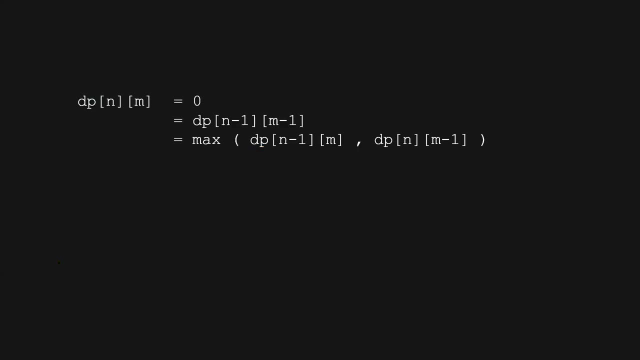 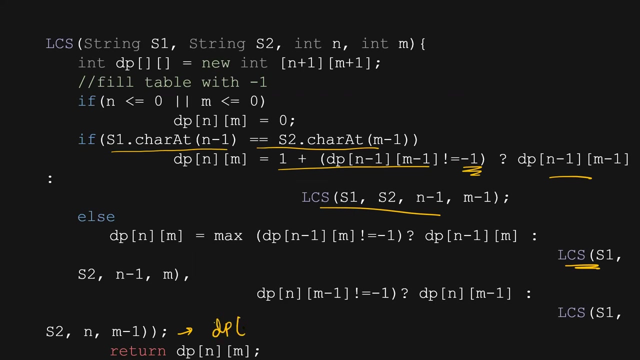 check whether it's already computed. if not, compute it, just like our previous algorithm, and store it. so we need to store it as well. before returning, store it into dp table. as i said, before returning, store it into dp table. whatever the value comes, you just store it. 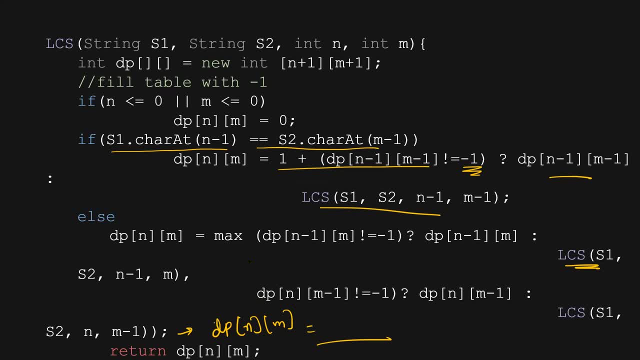 the max of this got it? that's a fairly simple ask. this kind of solution of dp is called top down solution, in which we are using recursion and also we are using table. so to avoid recursive solutions we are storing them beforehand. only now there is a different kind of solution which is called bottom-up solution. to understand bottom-up, 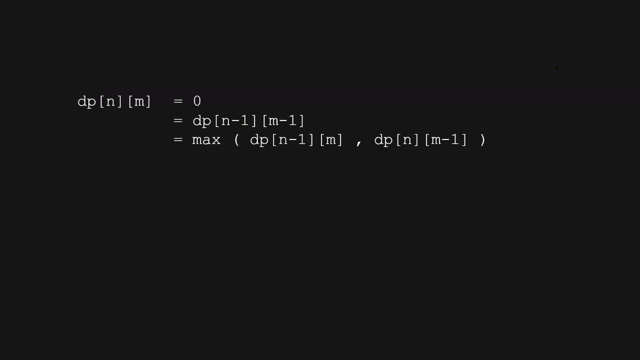 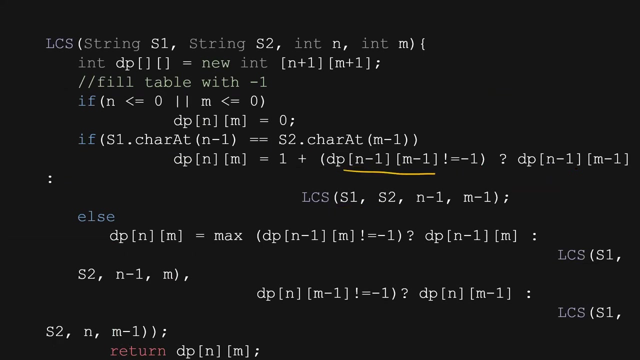 solution. what we'll understand is how this table of dp will be filled with this equation. it will be filled either dp of n minus 1, m minus 1- it is coming just from here, if we see, i'll just erase everything. so either a dp of n minus 1, n minus 1, it is coming. 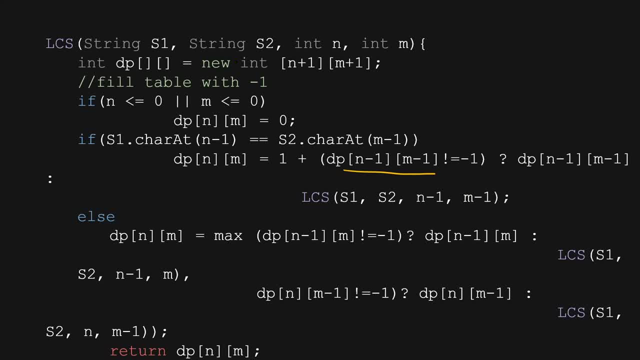 or we are recursively storing and storing, recursively calculating and storing and again returning. or dp of n minus 1 m, or dp of n m minus 1. we are returning. well, the près method for this is pretty simple. we are not disorting this table from the 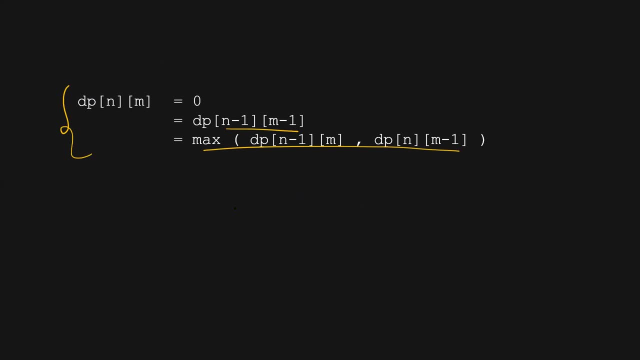 from the calculation which we carry forward from previous. so in a simplistic example, this one, this 2, can be my. so can i fill the table from beforehand? only something like this. let's say, i represent 0 0, 0 like this, and what i start doing is i check whether in an 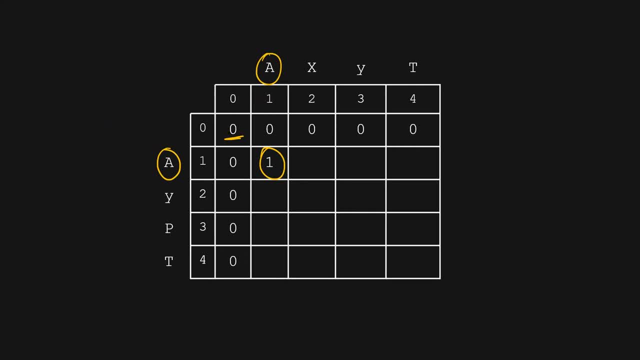 Obviously, if the length is 0,, nothing is matching, I stored 0. A is not compared with anything. then obviously the length is 0, is mute And obviously in the same way, if A, Y, P and T is not checked with anyone else, I am. 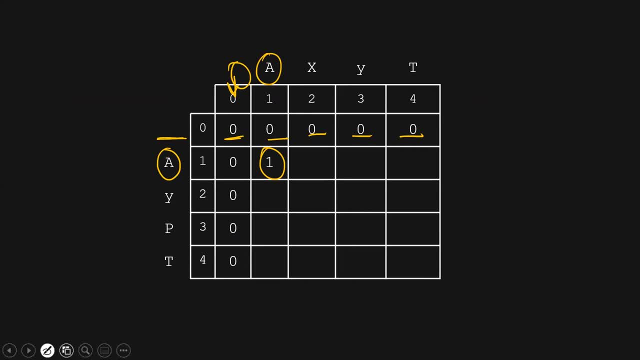 storing 0.. Now, further, I will start checking or creating a solution. If the string of index i and j, which is 1, 1,, if they are matching, I will store 1.. 1 plus 0 of that, which is like this: 1 plus previous, 1 plus 0, if they are matching. 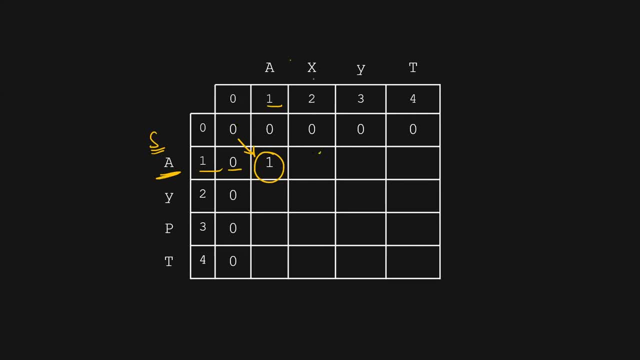 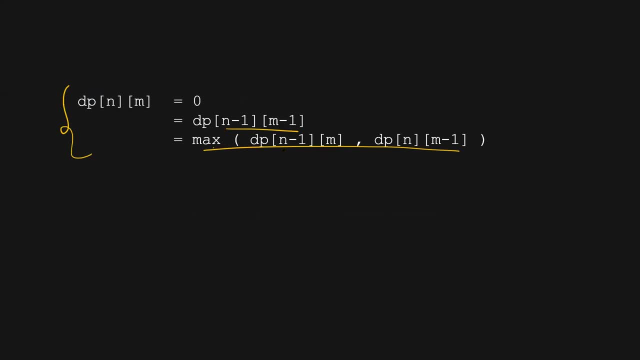 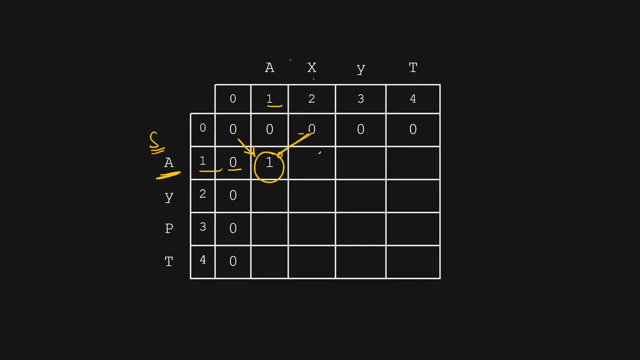 If let's say A and X are not matching A and X, they are not matching right. What I can feel, The max of DP of N minus 1 M or N- M minus 1, which is maximum of these two? Maximum of these two is 1.. 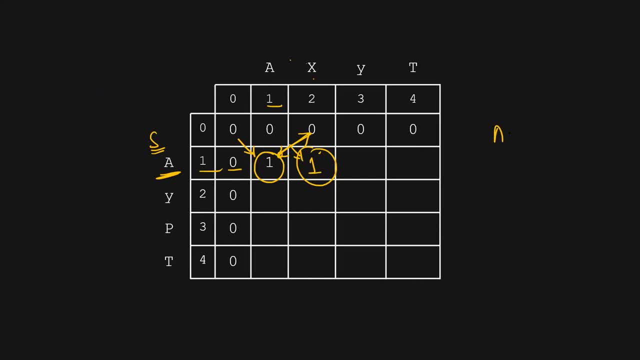 So that means when I am storing 1 over here. that means what Maximum of substring between A and AX is of length 1, which is A. Now, same way, A with AXY is also 1, maximum of these two. 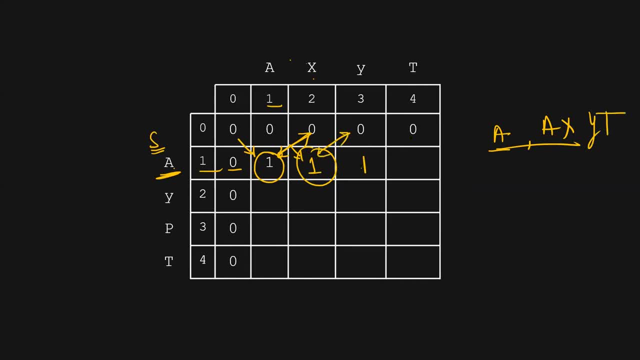 And AXY is 1. And AXY is 1.. And AXY is 1. And AXYT is also 1, maximum of these two I can fill it up simply Now again, I will process further with the length or the row 2.. 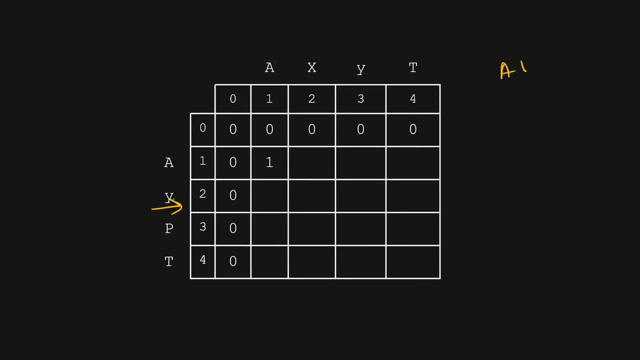 Again, I will check if Y and A is matching. that means I am checking if AY and A. what is the maximum characters that are matching over here? That is maximum of these two: 1, which is AA. Then for this the value will be AY and AX. 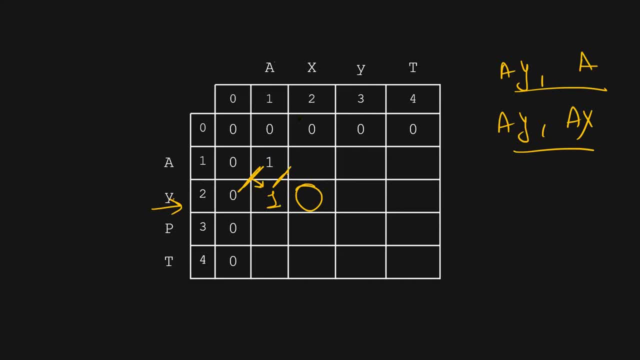 What is the maximum of these two? So Y and X are not matching, So maximum of these two, which is again 1, which is AA Now, if we see so value over here, will be 1.. So far, 1.. 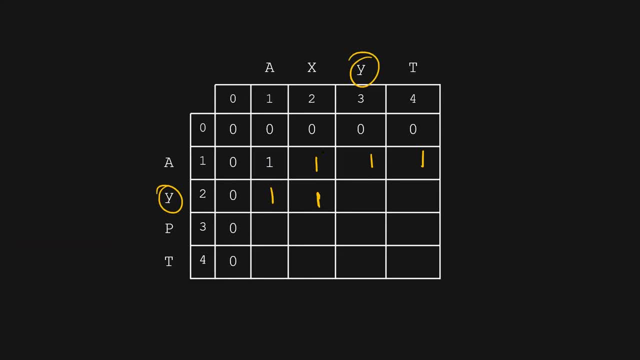 Now Y and Y are matching. What is the solution for that? 1 plus N minus 1 M minus 1.. 1 plus N minus 1 M minus 1.. So this represents that, But AXY and AY. what is the maximum subsequence matching in these two is AY, AY, which is. 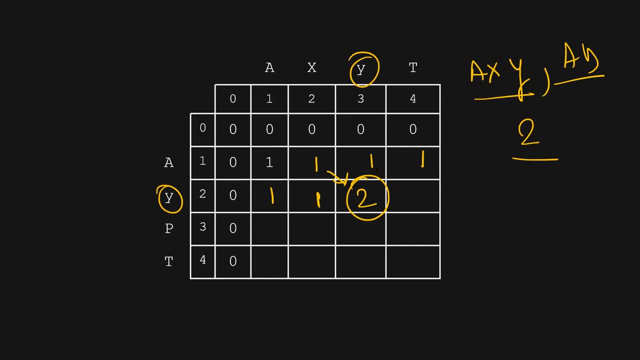 two length, which is represented by D, And again I fill up the same table. furthermore, as I showed, And at the end, 3 is coming. So DP of N minus 1, M minus 1 gives me answer 3, which is maximum subsequence in these two. 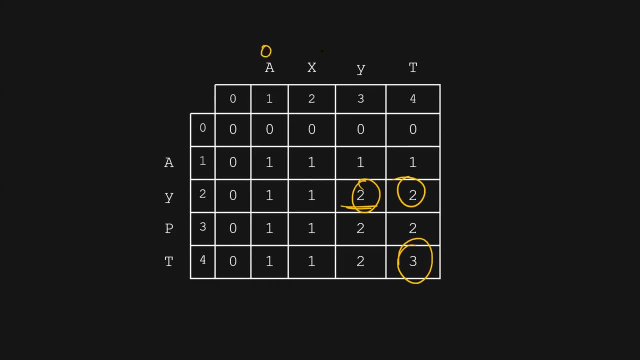 strings of character or length. 4 is AXY. I can fill it up with the same logic which we discussed over here. but I can fill it up the table beforehand. only I don't have to go in recursive solution, I just can do mathematically as well. 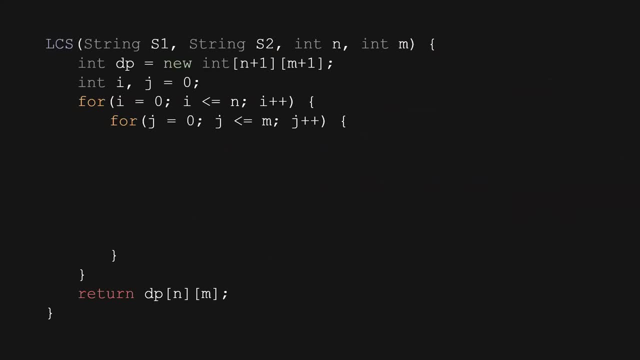 Now if you write down the code for that to fill it up the table, it can be very simply like this: That going into 2D matrix For I equals to zero to I less than N. J equals to zero to J less than N. going into 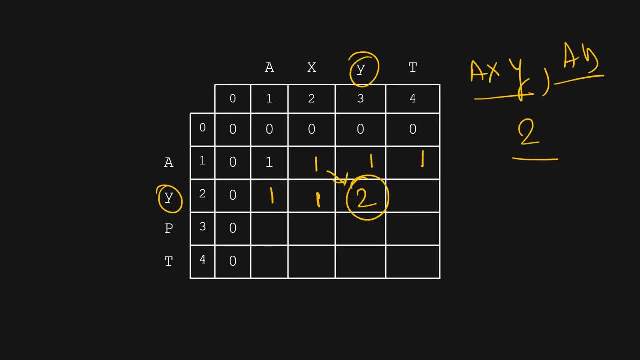 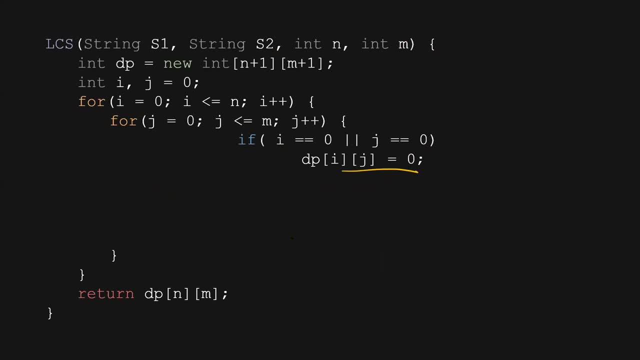 2D matrix row: wise, And the same calculation that we did over here, the same one. If I equals to zero, J equals to zero, store the value equals to zero For this row and this column, simple. Furthermore, if character at I and character at J are matching, the value will be 1 plus. 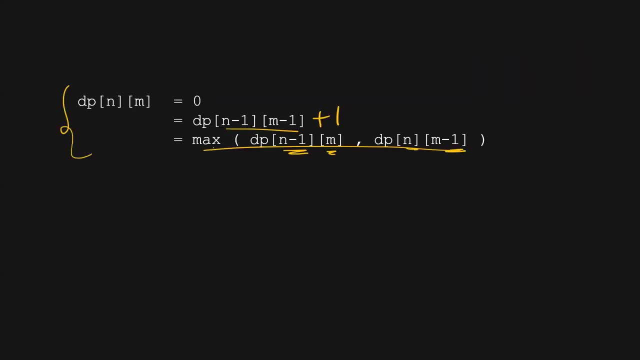 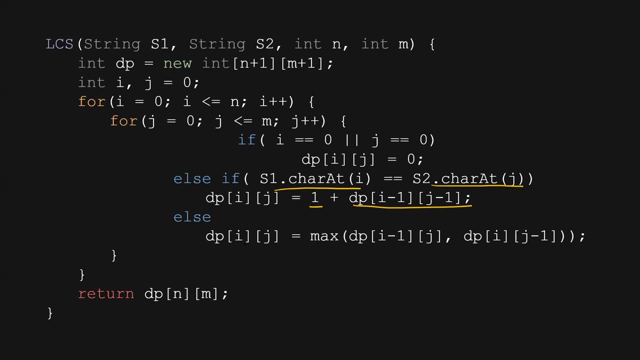 DP of I minus 1, J minus 1.. This one, N minus 1, M minus 1.. The same in terms of IJ, I minus 1,, J minus 1.. Else, if it is not matching the maximum of I minus 1, J or IJ minus 1, which is this recursive? 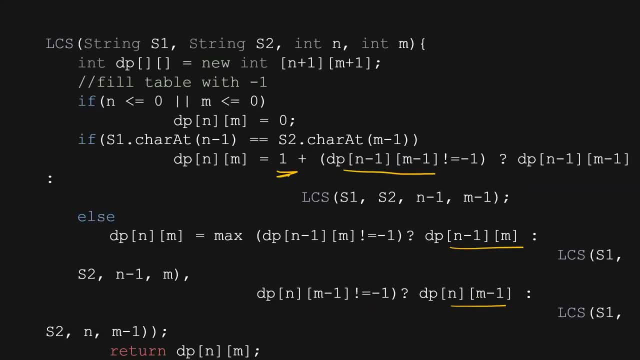 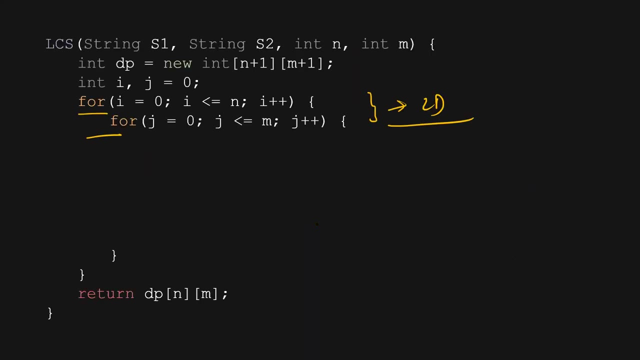 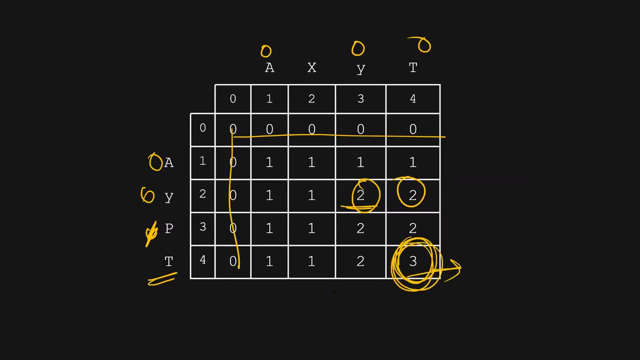 solution: I, J minus 1 or J- I minus 1, where it is this way, I minus 1, J, simple. So the same recursive solution I have converted into Bottom-up approach and I'm filling it up And at the end, whatever the last result comes, that is my solution. DP of NM. 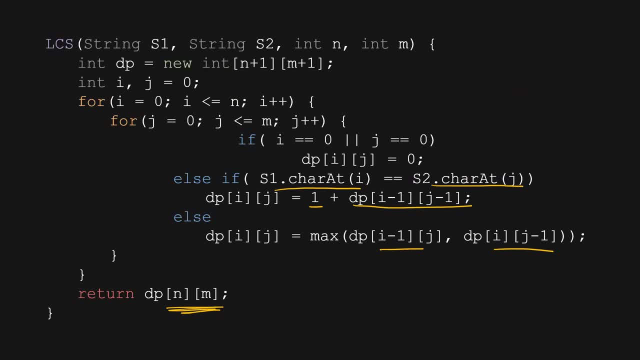 That is my solution. So in this way I can fill it up from the tabular's perspective. So you see, DP is not tough, it's just we need to create a solution from the base. Once we created a solution from base, 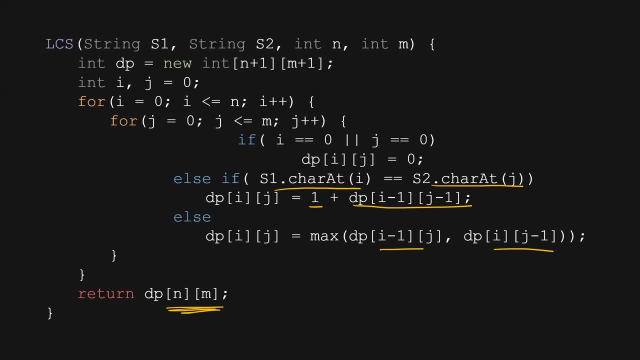 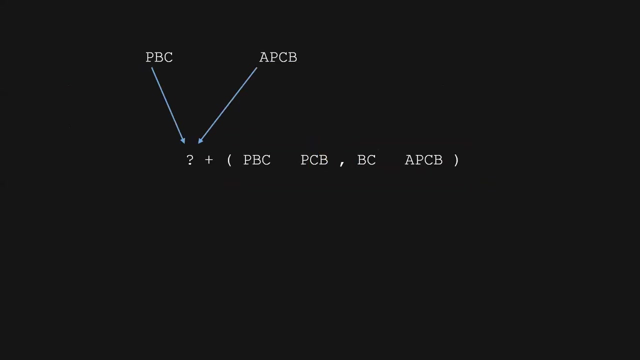 Storing it Into Table. Recursive formula Is easy, And converting that recursive formula into table is also again easy if we see similar recursive formula, only it is using. but the fact of is, or the essence of is, is that you need to create a solution from a very basic steps. 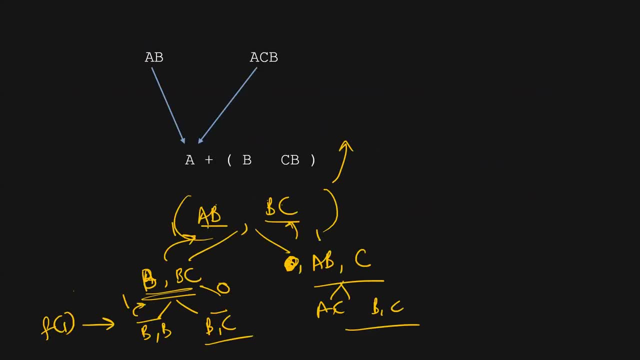 But if for one length string, two length string, it is solving for one length and two length, If recursive formula is solving for one length, two length and some arbitrary length, N, it is my final solution, a mathematical one. And then I created on top of that everything. 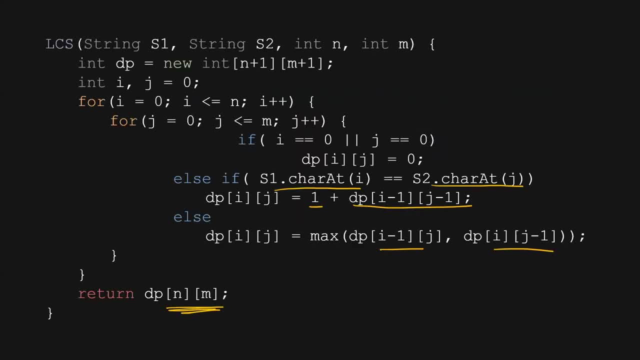 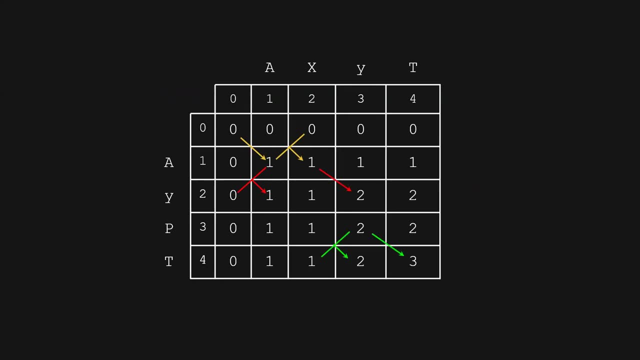 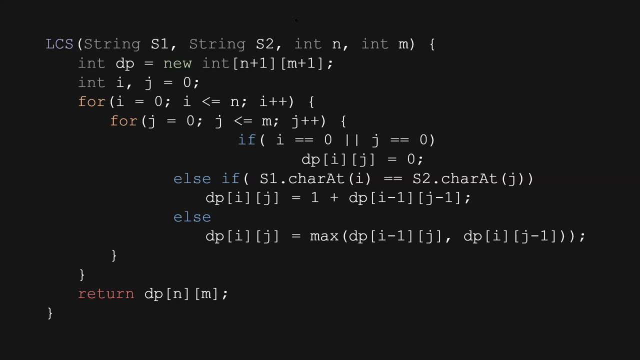 So far clear. So, as we saw, we filled it up like this: The table Is the table, So we have not solved it yet. Yeah, Any doubts so far. So with this practice, what we have seen is how to think in dynamic programming. 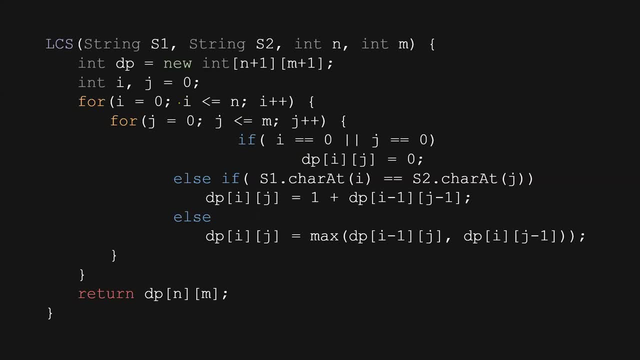 Now with further sessions, if it were to happen. what we will call it is for each and every data structure, If you join for that sessions with each of the data structures, how we should Make the steps, how we should build up such solution from scratch. 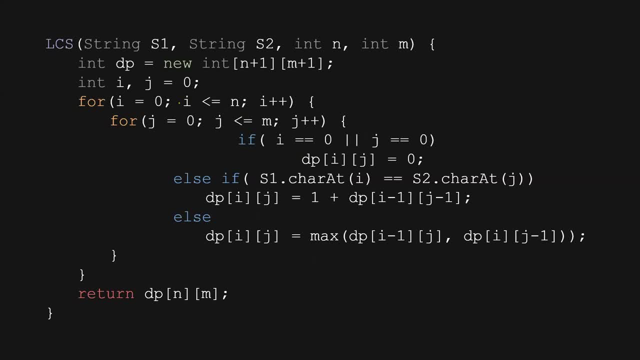 array linked list tree, try stack queue, heap, hash map, red black tree and try then graph, then 2D metrics and then with that programming how we should think and create solution from base- in interview as well. 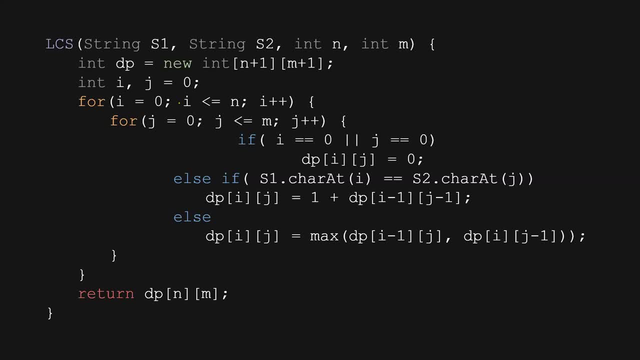 so that you don't have to bug up any solution. This is what our end goal is to teach you guys. Furthermore, I just want to give you one logic, which is: do you see optimization in this? So in interview, they will ask you something like this: 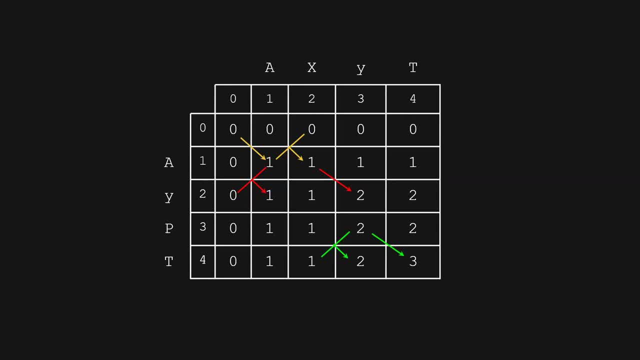 Okay, you created a solution from scratch. Let's say you didn't know, but you could create the solution from the scratch in interview. Do you see some optimization into this? Any guess so far? Well, just by seeing the 2D metrics. 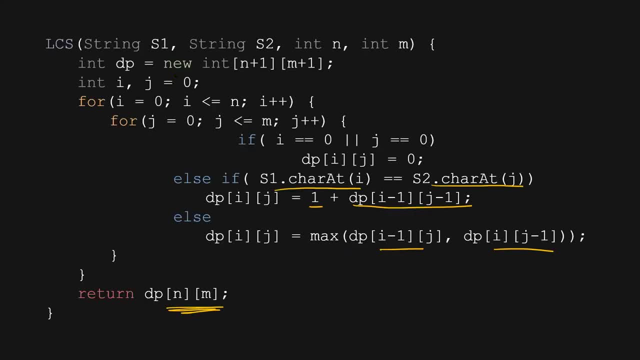 No, I'll give you a hint that if we see at any given point of time while filling up the table what rows are required, Either last row, last column or last row, same column or same row last column. So if you see, 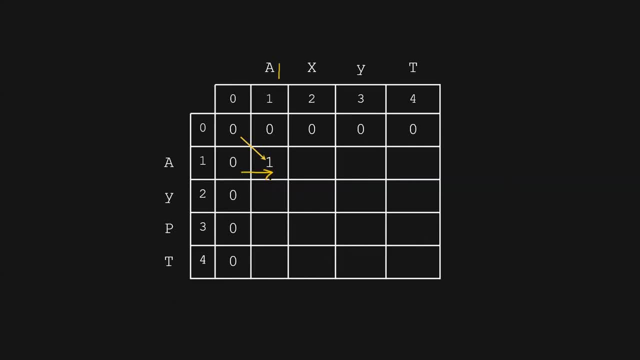 while filling up a column or a row like this, I just need either the same value. So example: let's say, while filling up this, I need the previous row or previous column. That's it Same way when I was filling this one value. 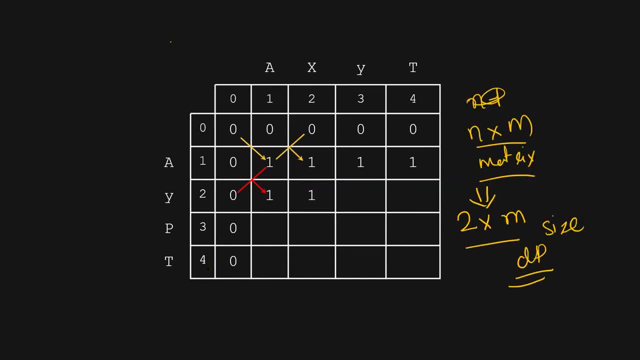 what I need: metrics in DP solution. So in an interview when they ask you any DP question, they will think that you should solve with the least possible space utilization and the least possible time complexity. generally recursive solutions are in exponential time complexity and exponential 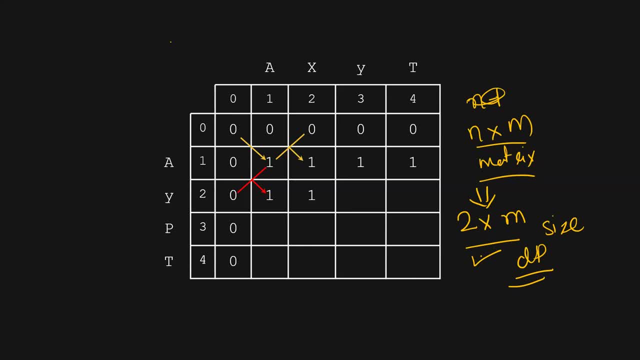 space complexity, but the optimized dp solutions will be maximum into order of n square time complexity and order of n square space. complexity is the least in dp generally goes, but still in space complexity if you can utilize like this, it is advisable. so can anyone think how can i convert this solution? 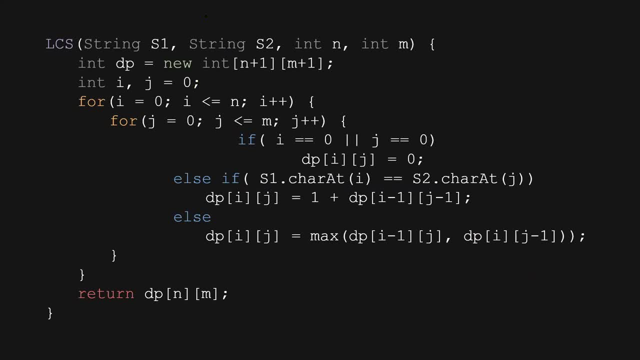 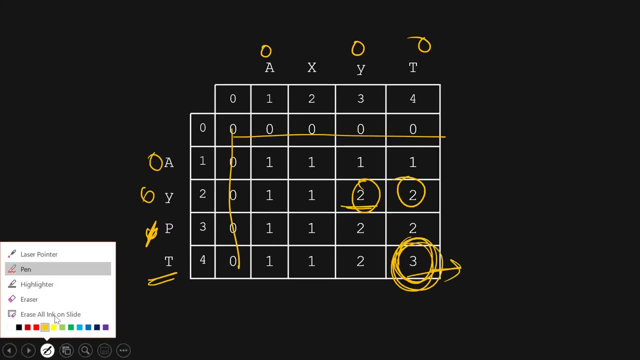 to two rows or two column level solution. it's fairly easy, as i said, that if you see at any given point of time i am using either of these three value, let's say to fill up one, i am using either a previous row- same row, previous column, previous row previous column or previous row same column. so if i say 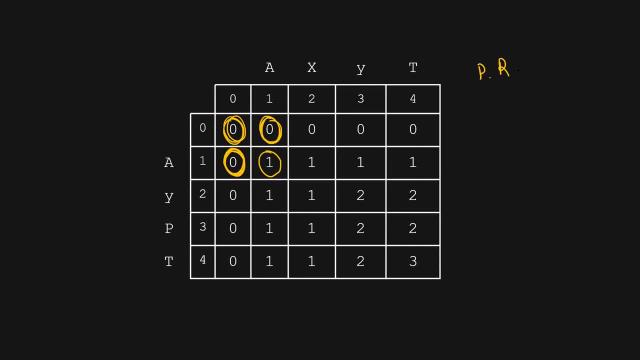 previous row, same column. previous row, previous column, or same row, previous column. so these are the things that i'm using. either of these three i'm using at any given point of time, let's say while filling the cup of this three. also, i use this two plus one, three, which is like previous row, previous column. 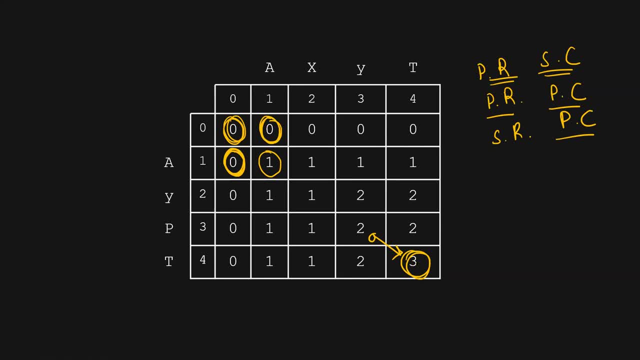 so what? i'll do that while filling up with this three. i don't need any of this row, right? can i reuse those rows just for mathematical way? so if i use something like this: that index is zero will represent index zero. index one will represent index one. now to fill it up: the values of index two at the time of two: what? 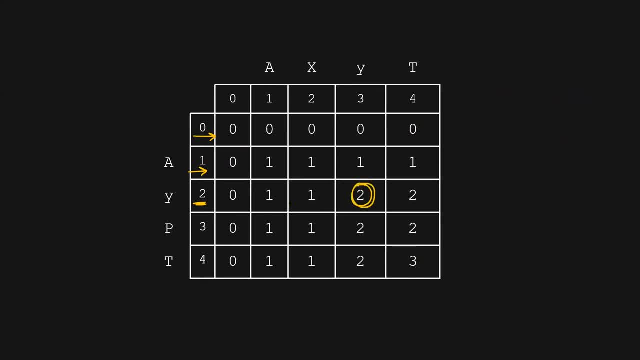 i need, let's say, to fill it up to what i need, the same row and previous row, right, so that i'll fill it up in the unused index of zero, because now, if you see, the zeroth index value is never being used by i'm filling it up for index two. so at index two i'll reuse the column of zero and fill it up. 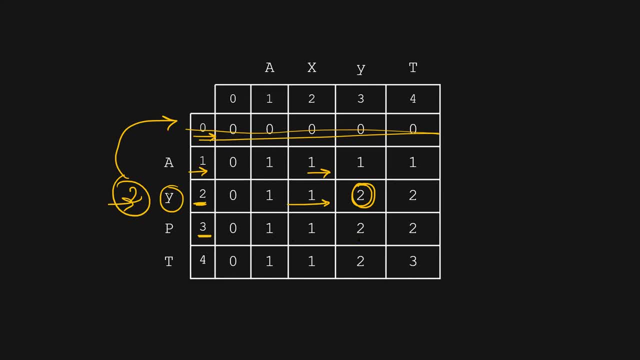 while filling up the value of three, what i need? third row and the second row. second row is being stored at what zeroth? now, if you see first index is not used, so three, third index row, i'll use it for first index. so if you see, i'm just using any index. 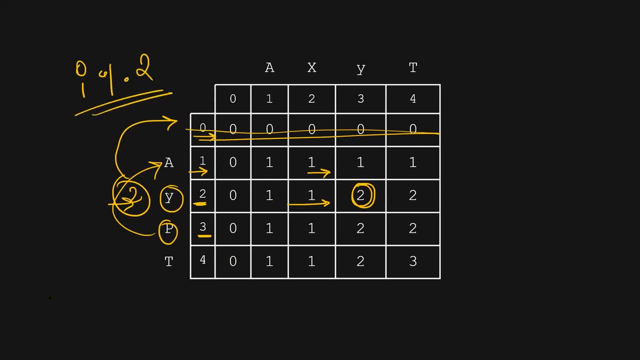 row five, modulus or percentage two. percentage two in the sense a mathematical one, expression one, but modulus two, i'm using it. so index two actually is being stored at index zero and three is being stored at one, and then i can reuse that and i can reuse the whole. 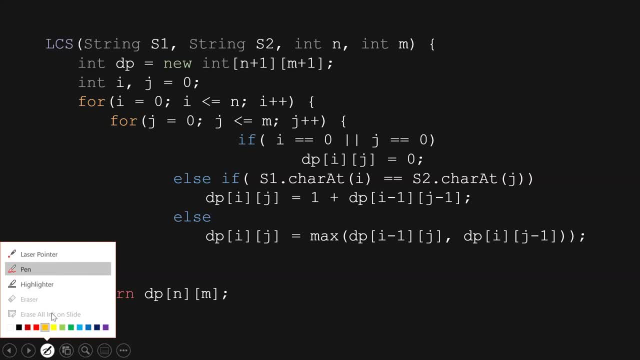 solution very simply like this: that instead of creating n cross n plus 1 cross m cross m plus 1, i'll create a solution with 2 cross n plus 1.. with 2 cross n plus 1, i'll create a solution with 2 cross n plus 1.. 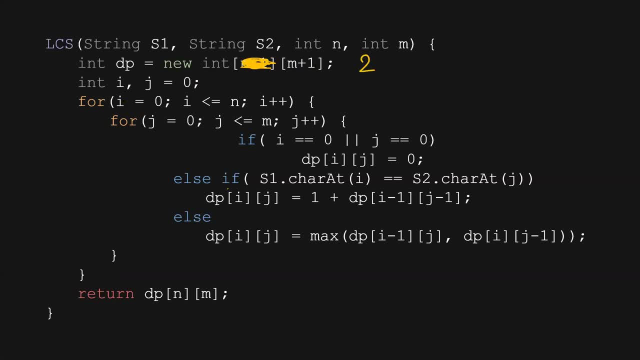 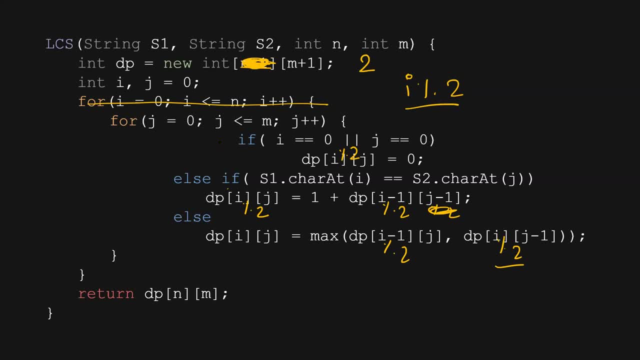 and every time i have to replace the i, so that's why i will equals to i and and 2. that's it. in this way, my whole solution of working one is converted from n cross m to 2 cross m. you can try out both the solutions, this one which i say. 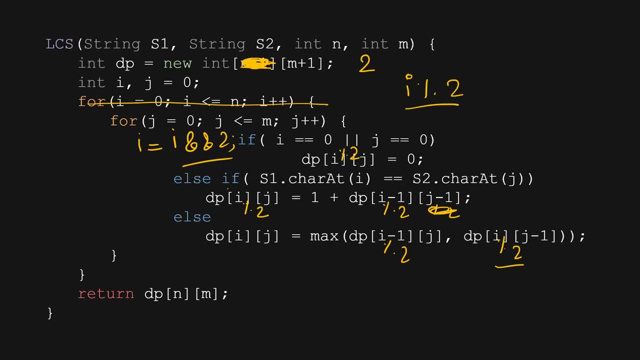 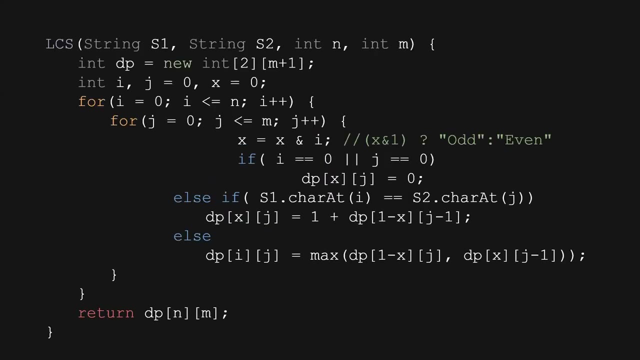 you can convert this in into code and you can see whether it's working or not. and the second one, which is with having a two rows, only got it. so if i have this, i have the solution ready. so, if you see, i'm using four loops, same way, but the created of two length only, and instead of i i'm using x, which. 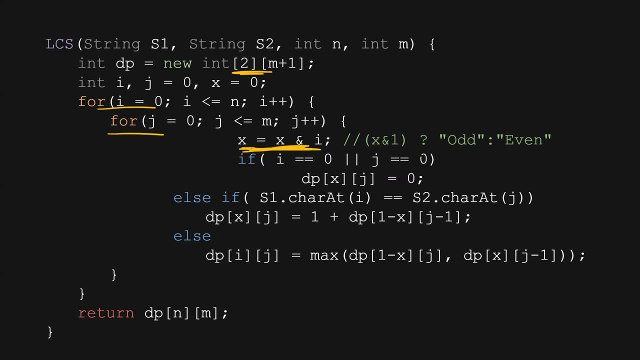 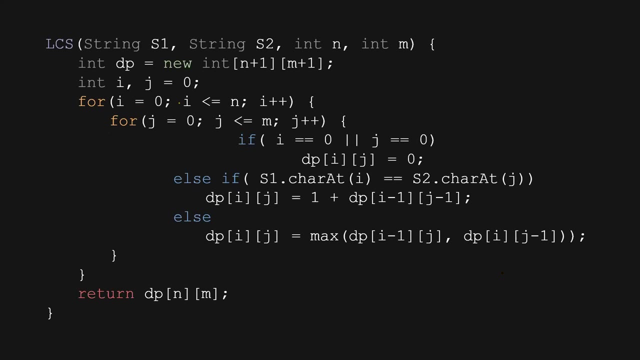 is with modulus 0 and 2. so x and 1 will give me either odd or even values, and by that, instead of modulus 2, what i'm using? x only. i minus 1, x, 1 minus x- the same solution i'm using, if you see. 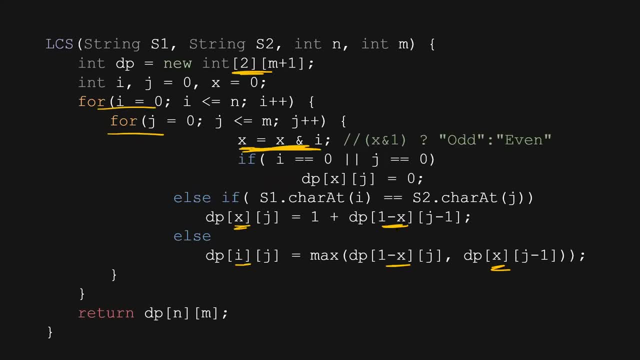 just one difference is there: over here it's i minus 1, over here it's 1 minus x, y. because i don't want to do like x minus 1, because x can take 0 or 1 value, so 0 minus 1, minus 1. i don't want to do in matrix, so that's. 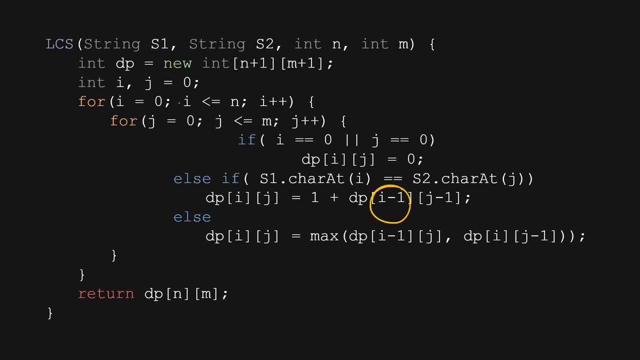 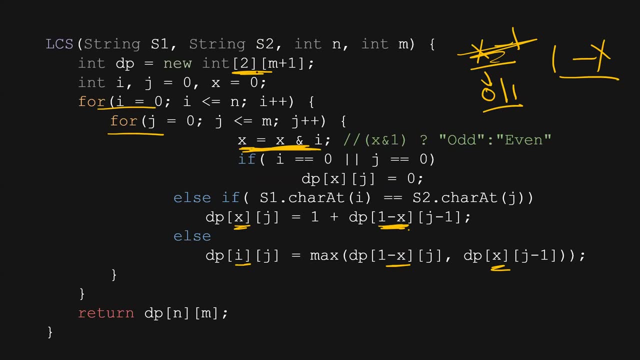 why what i change to 1 minus x, that's it. apart from that, no change. so with this i have least optimized solution with dynamic program for longest increasing subsequence and, as i said, the variations of longest increasing subsequence we have taken in that way people will ask it didn't into the interview, not directly- that solve longest. 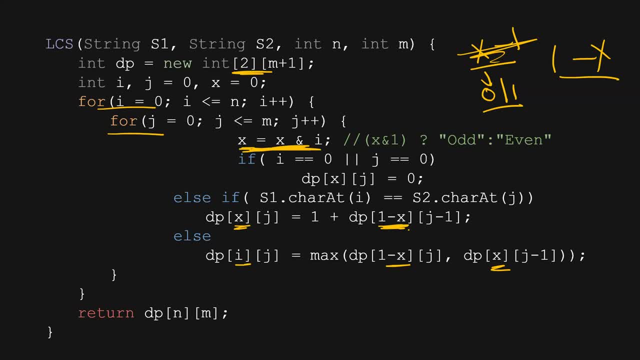 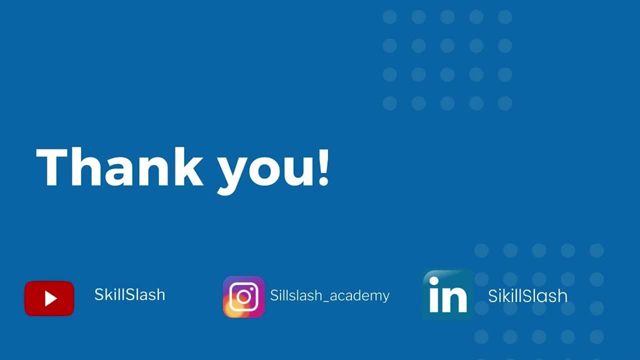 common subsequence, but they will give some variations of longest common subsequence and they will ask: 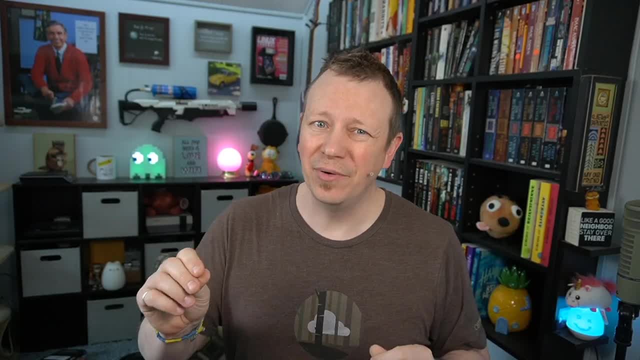 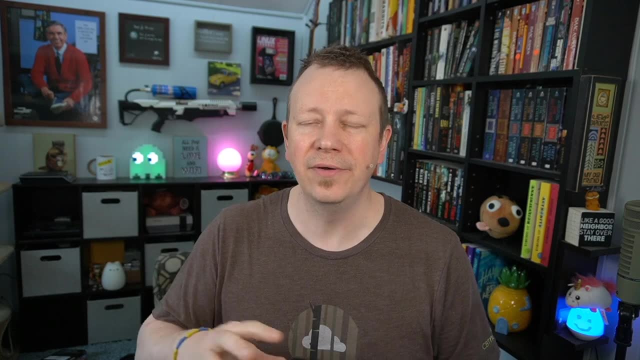 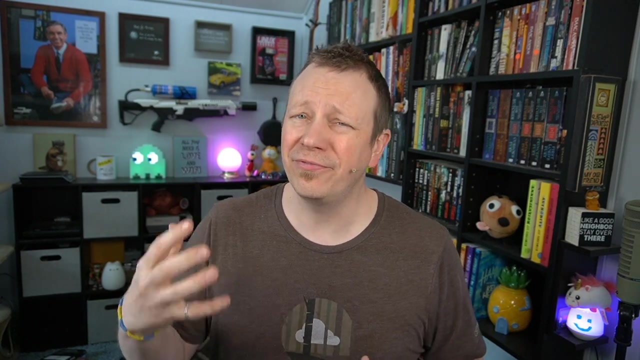 So everybody knows that backups are important. However, backing up live databases takes a little bit of nuance because the files are constantly in use. Now, with databases- today I'm specifically talking about MySQL and or MariaDB. Now they're functionally very, very similar MariaDB actually.